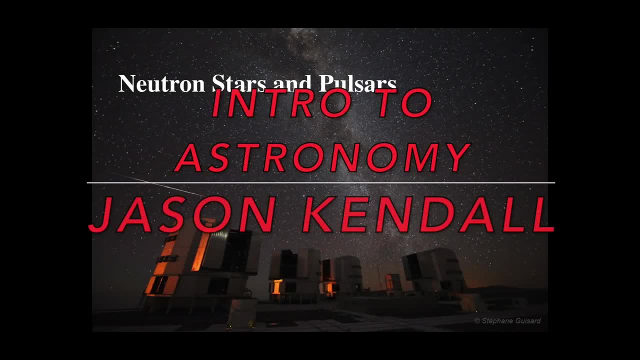 Hello, this is Jason Kendall, and welcome to the next of my introductory astronomy lectures. This time we're going to be talking about neutron stars. neutron stars and pulsars. These are the massive cores of massive stars after they have died, So this is an amazing set. 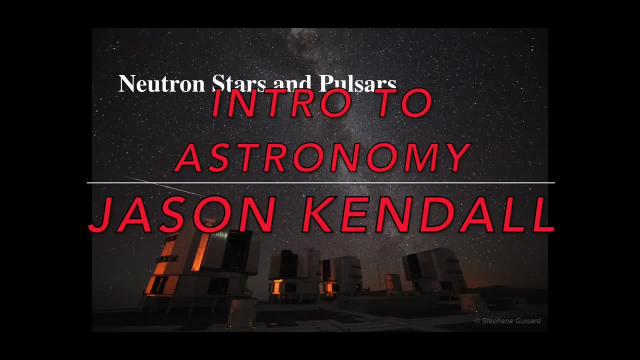 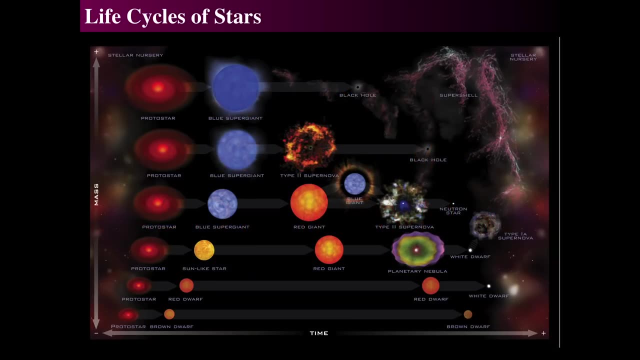 of things. Last time we talked about white dwarfs and what they can turn into. We only said they were the low mass or medium mass stars, but now let's look at the ultra rare type stars and what they do. So once again, let's go back and look at our life cycles of stars thing We have basically. 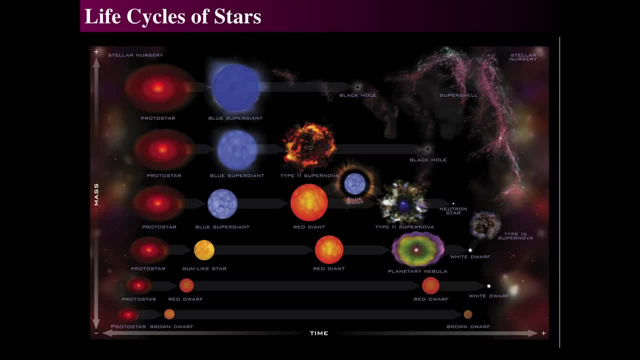 six layers that we talked about. At the bottom are the lowest mass stars, which are barely, barely, barely stars at all. They're effectively not even stars because they don't even do nuclear fusion in the core. Those are the brown dwarfs. Red dwarfs are the G and the K and M type dwarf. 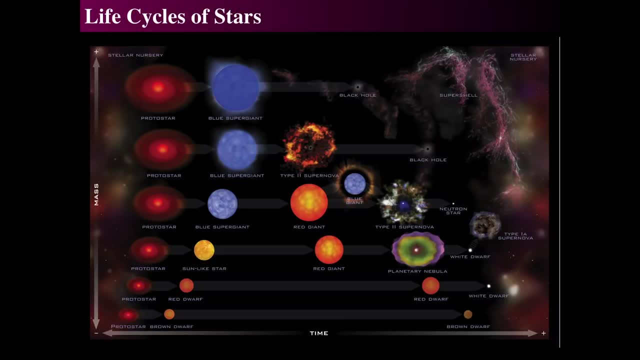 type stars. They just burn for up to a trillion years and then eventually become white dwarfs and just fade away into obscurity. Something like the sun or a little bit more massive The sun between, to say, the sun's mass and up to about eight solar masses. A sun-like star will live a few billion years. The sun will. 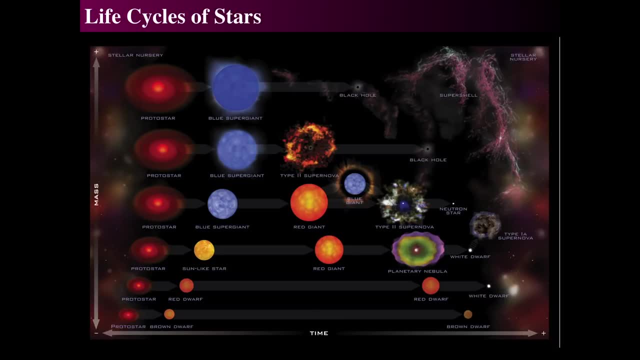 live 10 billion years. More massive stars live shorter. They become a planetary nebula and make a white dwarf And if they're in a companion, do a supernova. But now we're going to be talking about the next level up, much more massive stars, stars more massive than the sun that then turn. 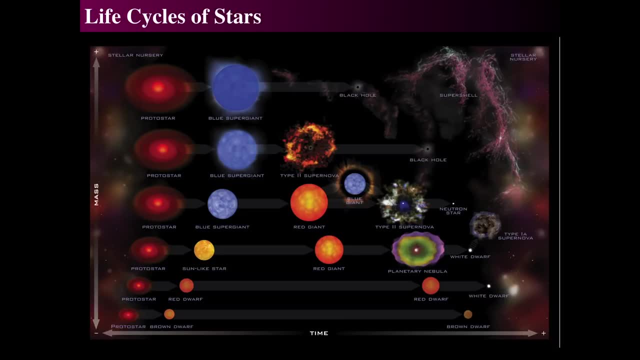 into giants, and then blue super giants, and then explode into a nova, which we talked about last time- supernova explosion, And now we're going to see what the remnant is: a neutron star. And that's what we see in this thing. The other two things we'll talk about next time, All right, So 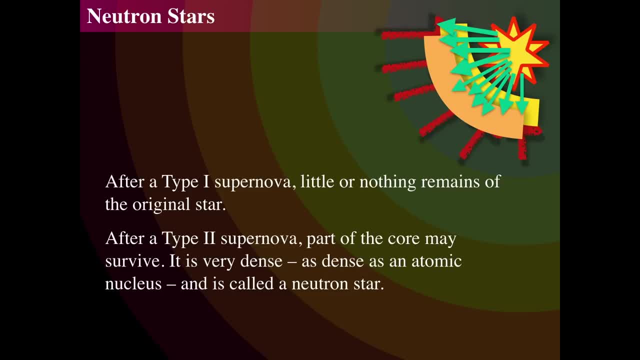 neutron stars after a type one supernova, which is a white dwarf, having so much stuff that piles on top of it that it explodes under the Chandrasekhar limit. A type two supernova is a supermassive star that gets compressed down into the core and that core material then becomes a 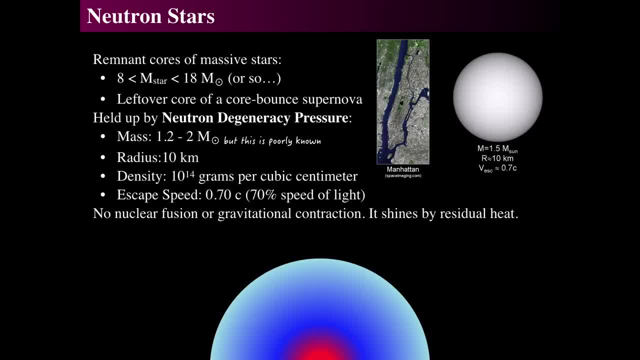 neutron star. And what are neutron stars? They are the remnant cores of supermassive type stars. Well, supermassive meaning eight to about eight, or somewhere between 10 and 20 solar masses as the original star. And when the supernova occurs, there is a bit of a leftover piece, Remember we. 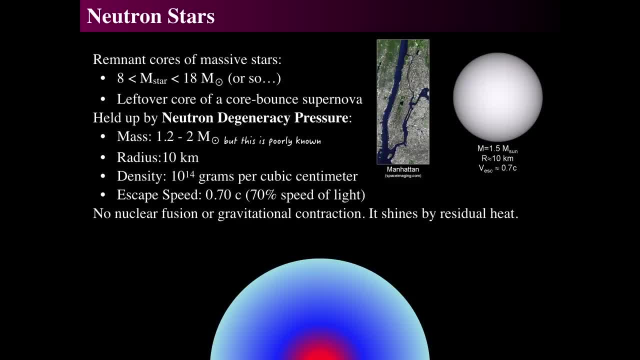 said in the supernova lecture that there's a core bounce as everything gets to be this incredibly high density down in the core during the supernova. So this thing that happens is they get compressed so incredibly tensely that we are now, instead of having electron degeneracy, which we talked about in the previous lecture, now we have neutron. 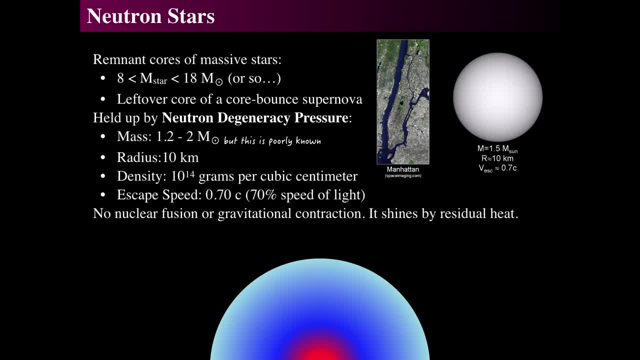 degeneracy, And so this is the same thing as electron degeneracy, except it is done with neutrons. So instead of the electrons holding it all up and just kind of, and their pressure is no longer dependent on the temperature, now the neutrons and the electrons and protons merged. together, And so this is the same thing as electron degeneracy, except it is done with neutrons. So instead of the electrons holding it all up and just kind of- and their pressure is no longer dependent on the temperature, now the neutrons and protons merged together to form neutrons, And then those 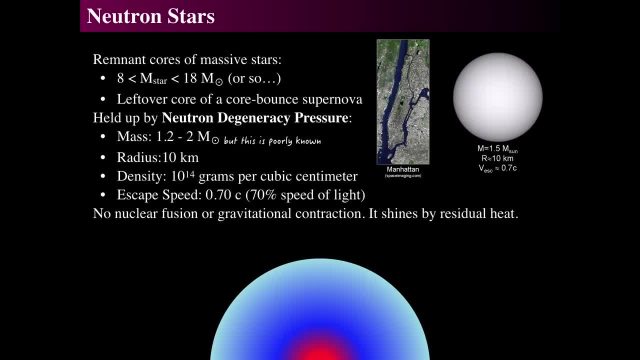 things then support the entire mass of the star. What's left of a stellar core from a star that originally was between eight and 18 solar masses? the rest, the remnant, is between 1.2 and about two solar masses, but it's really not well known. The radius is about 10 kilometers, which is very small. 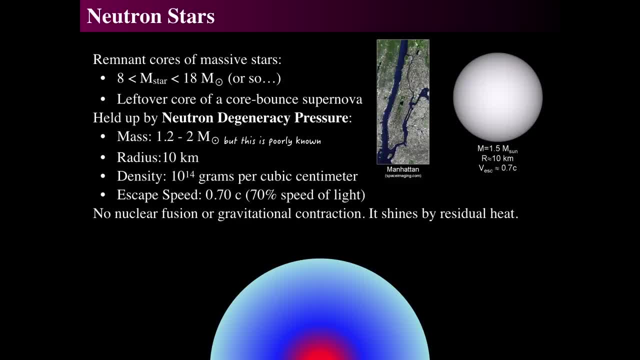 And the density is enormous, about 10 to the 14th grams per cubic centimeter, which is gargantuan. Funny thing is, is that something? that's that massive, two solar masses compressed down to 10 kilometers? the escape speed then is really big, about 70% the speed of light, and it has amazing 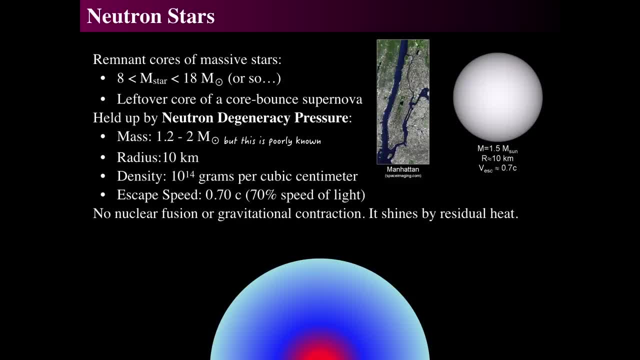 amazing, amazing results. And there's no nuclear fusion happening in this thing or any gravitational contraction. It is being held up by the neutron degeneracy pressure. It won't contract under gravity anymore because that pressure is holding it up And there is. 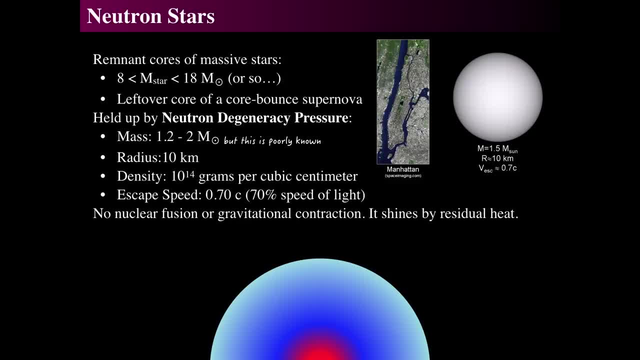 even though the effect of the electron degeneracy is not so great. it's not so great, it's not so effective. the temperature is extraordinarily high. there is no longer nuclear fusion occurring in it, And so there is residual heat. that is that happened with this thing, and they glow with the residual heat. 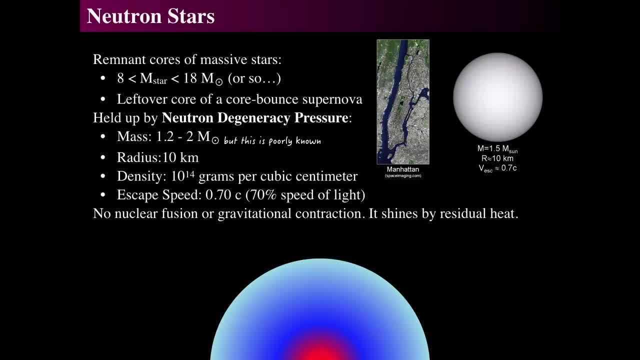 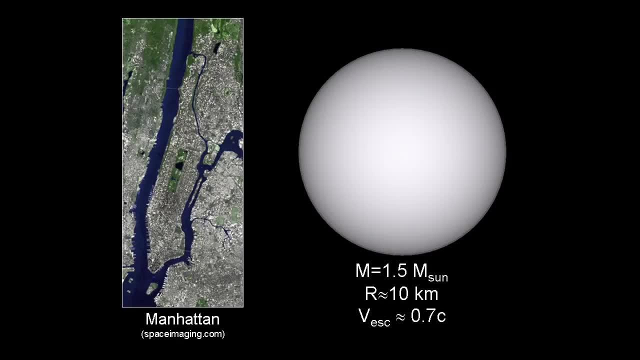 However, they're really tiny, so their luminosity is incredibly small. How small, Remember: these objects are about the size of the island of Manhattan, about 10 miles or so across, about 10 kilometers across, and say the mass is about 1.5 times the mass of the sun, which is about 10,. 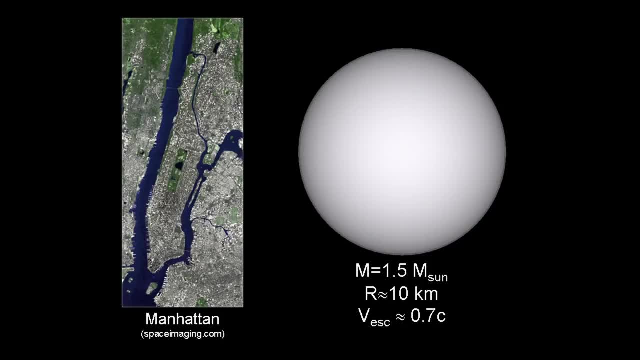 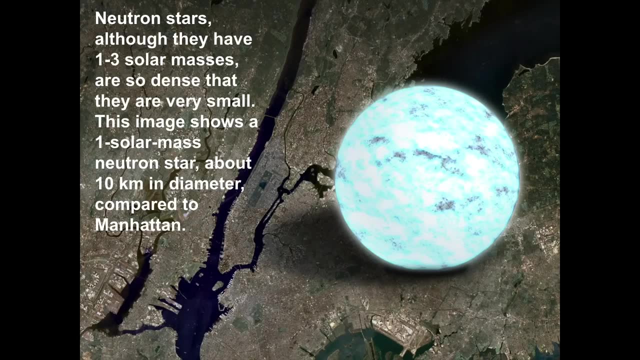 and that's an incredibly packed object. So, and the escape speed is about 0.7 c or about 70% the speed of light. So these things are tiny And they go through about 1.3 solar masses. They're. 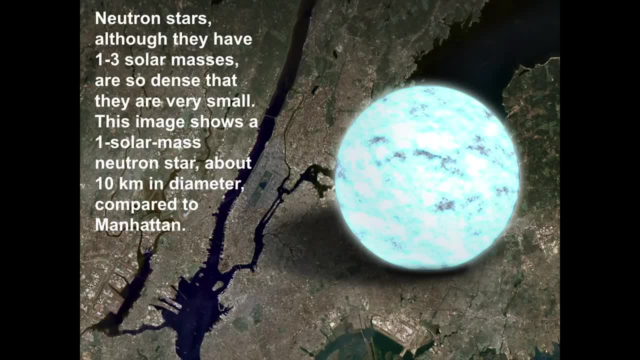 incredibly, incredibly dense. If a neutron star were to rest on top of Queens and Long Island, there wouldn't be anything left of the Earth. I mean nothing. There would be nothing, Couldn't hold it up. The Earth ain't that strong. It would be on the surface of the white dwarf. So if you 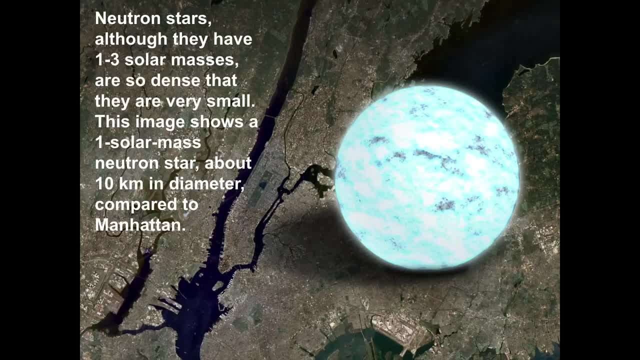 Google Discovery Channel and look at neutron star colliding Earth. you'll find a crazy, crazy, crazy video on Discovery Channel that shows what happens when a neutron star collides with Earth. Basically, the Earth becomes, falls onto the surface and is torn into shreds and becomes a skin only a couple of centimeters thick. 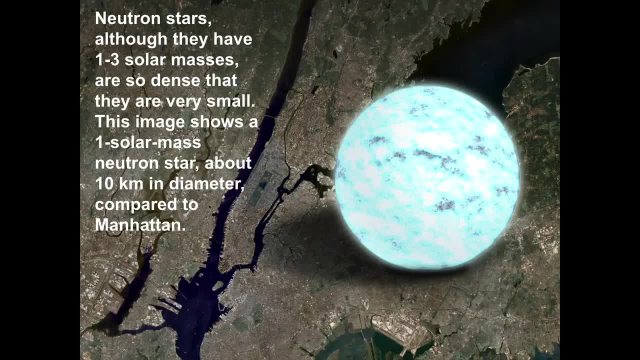 on the surface of the white dwarf. That's what would become of the Earth if this situation that we see in this image happened. That would be bad- Yet another of the million ways to die in astronomy. All right, So let's talk about the ranges of masses. for neutron stars, They range in mass. 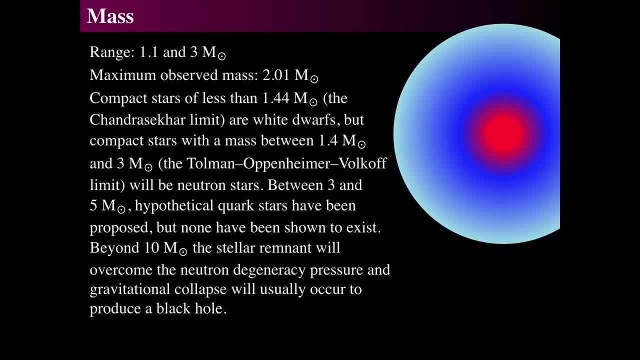 roughly between 1.1 and 3 solar masses. This is not incredibly well known, but that's the observed maximum mass. The theoretical mass is between 1 and 3.. But the maximum observed mass is about 2 solar, just a little bit over 2 solar masses. And remember that any compact star 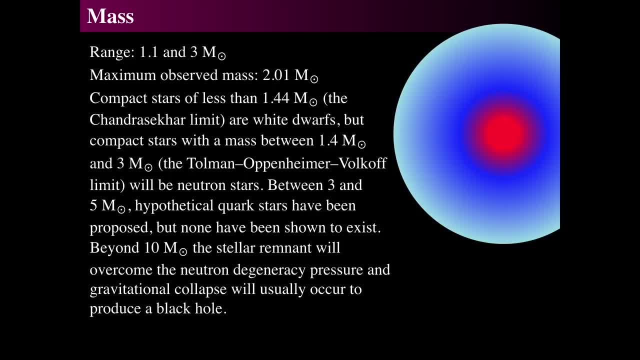 smaller than 1.44 solar masses, which is the Chandrasekhar limit. the Chandrasekhar limit is the limit of electron degeneracy as the electrons get closer and closer and closer to the speed of light, And so once the electrons are moving at the speed of light, they can't support. 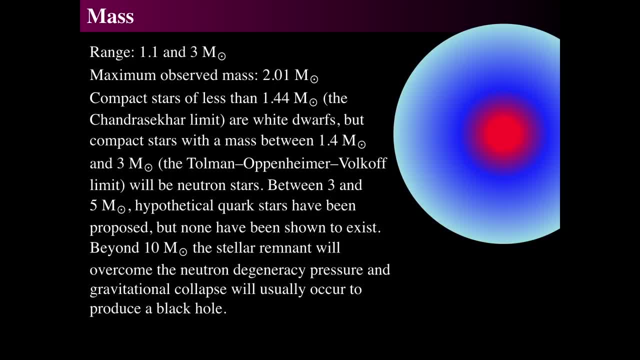 it anymore, because that's the maximum possible energy that they can have. So then the star is collapsing and collapsing, collapsing, and the electrons are moving faster and faster and faster. So that is the maximum limit that a white dwarf can have. However, 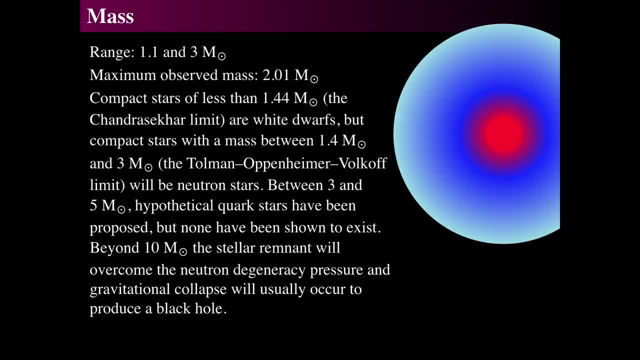 if they merge together they can form a neutron star. Now, if it approaches the Chandrasekhar limit as a white dwarf, it'll explode. But if the mass, if it collapses under the power of a type 1, type 2 supernova, then it can exceed 1.4 solar masses and go between 1.4 and 3 solar masses. 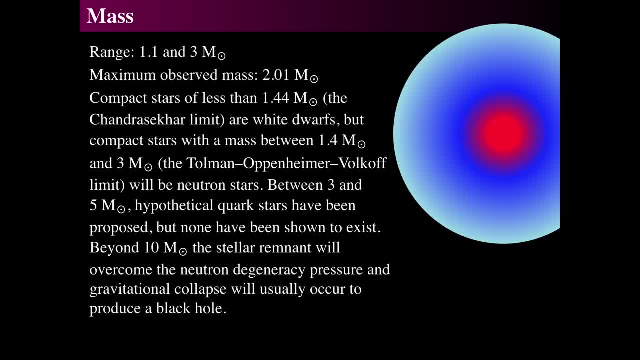 which is called the Tolman-Oppenheimer-Volkoff limit, which is a similar thing to Chandrasekhar limit, except now, instead of electrons, it's a white dwarf. So if the mass of a white dwarf is not electron degeneracy, it is neutron degeneracy. So go back and look at my really. 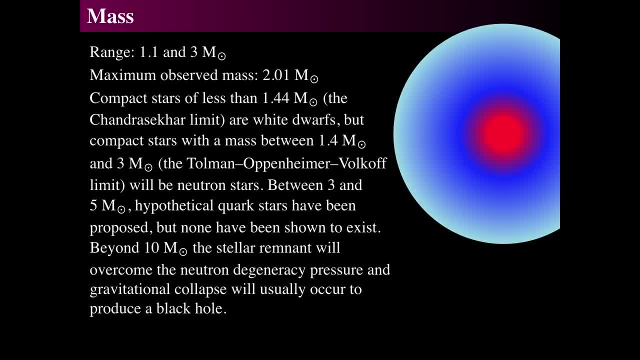 long lecture on the nature of electron degeneracy and the previous one on white dwarfs, to know what I mean by that. I'm not going to go over that again here. So neutron degeneracy is basically the same thing. It's a similar structure as electron degeneracy, except that the pressure 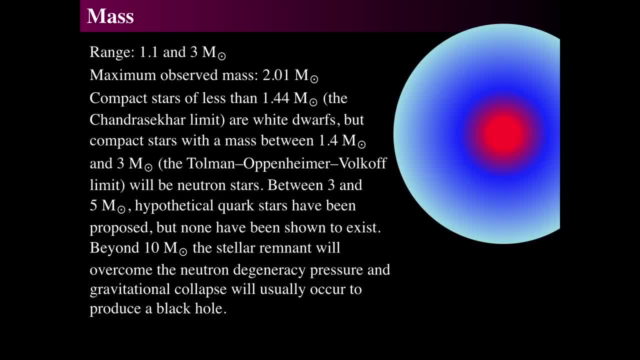 has been, is so high that the protons and electrons merge together to form neutrons, and that is the link that pushes them all together. So then there is: if it's above 3 solar masses, then the then it could be. there are other things that are potentially smaller than. 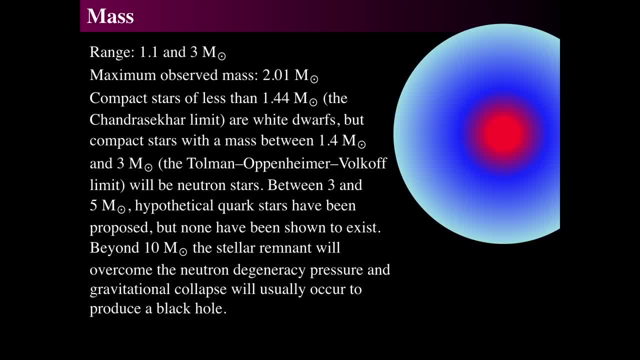 neutron stars and the neutrons can have maybe what we call quark stars, where it's not neutron degeneracy that holds it up, but quark degeneracy. And what are quarks? Quarks are the constituents of neutrons and protons. However, there are no, there's no objects that are known. 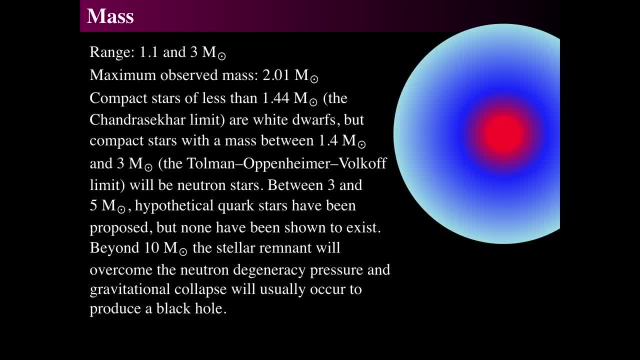 that could possibly be a quark star, because the maximum observed compact star is about 2.1, 2.01 solar masses. Beyond 10 solar masses, nothing's going to win and you have what's called neutron degeneracy pressure. No matter what, we'll lose and it will have to collapse. 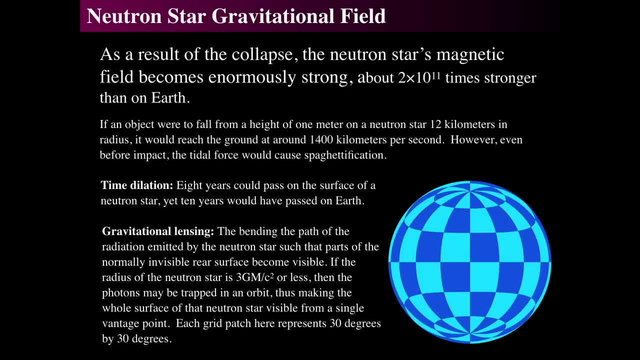 to a black hole. So let's see what that works out to be. But neutron stars. when they collapse down to these really, really, really tiny, tiny objects, the gravitational field becomes catastrophically large. The field is so big- it's over 200 billion times stronger than 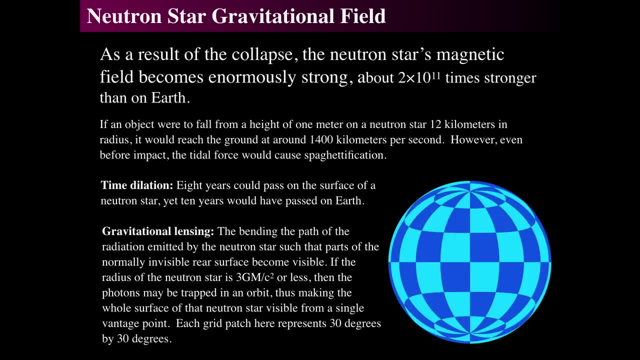 the Earth's gravitational field. Well, okay, oops, I made a mistake here, Got a typo. Actually, the typo is: is that the not the star's magnetic field, but the neutron star's gravitational field? It's insanely, insanely powerful, over 200 billion times. Remember magnetic fields. 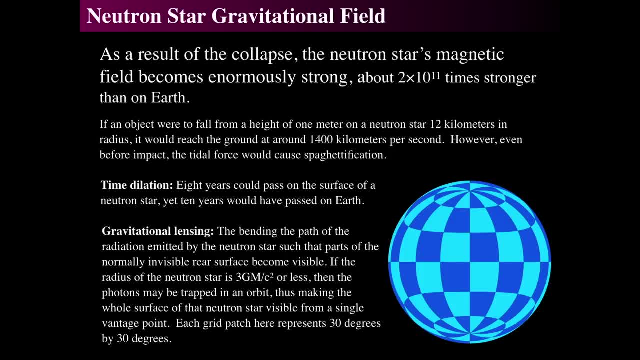 are different than gravitational fields. So if you're just looking at the words, you're going to see I have a mistake And I'm not going to stop this lecture just because of this mistake. I'm just going to keep going on because here we go. Should have got that at the beginning, but hey, whatever It's. 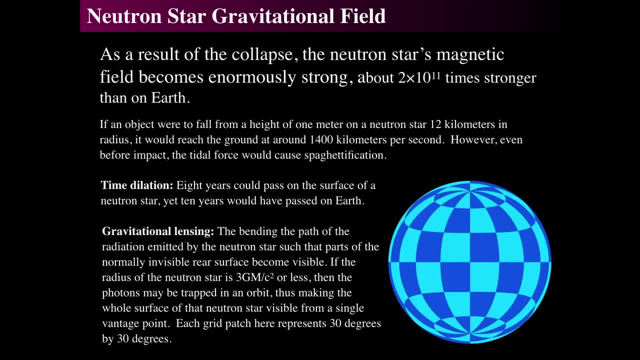 live theater right. So if the gravitational field is over 200 billion times stronger than the Earth, then nothing could resist the gravitational force of that and it will be smashed to a complete pulp. All the atoms inside it get ripped apart in very strange ways. 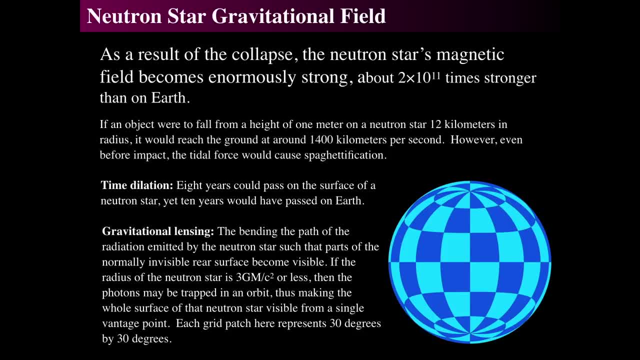 Michael Keaton. So if you had something on the surface of a neutron star Superman, well Superman wouldn't even make it. but let's say something was one meter above the surface of a 12 kilometer radius neutron star. if you dropped it from a height of one meter by the time it hit. 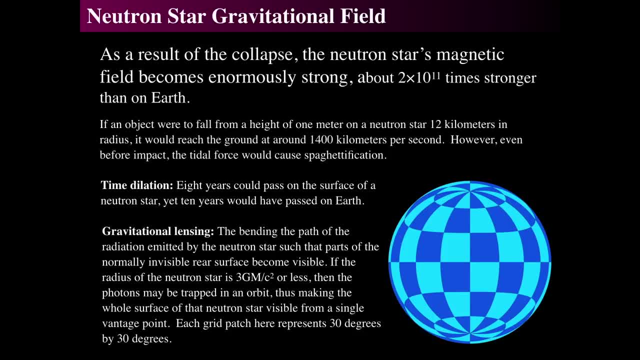 the surface of the neutron star one meter down, it would be going 1400 kilometers per second before it hit the ground. hit the surface, the tidal forces would stretch that thing apart whatever it is and would actually turn it into a spaghetti thing. So even if it was something as 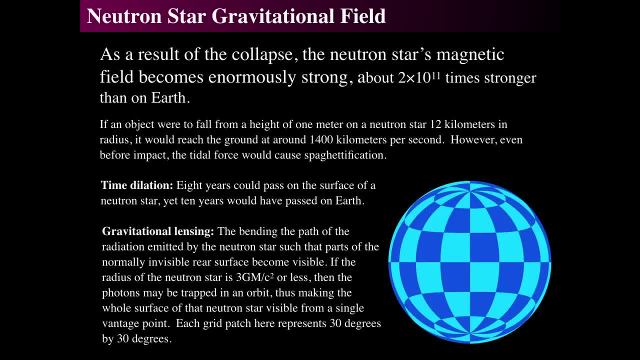 small as a golf ball. that golf ball would become a spaghetti string, meaning the top of the golf ball would be stretched away from the bottom of the golf ball And the force or the energy released by that would be greater than all of the nuclear bombs ever exploded on the surface. 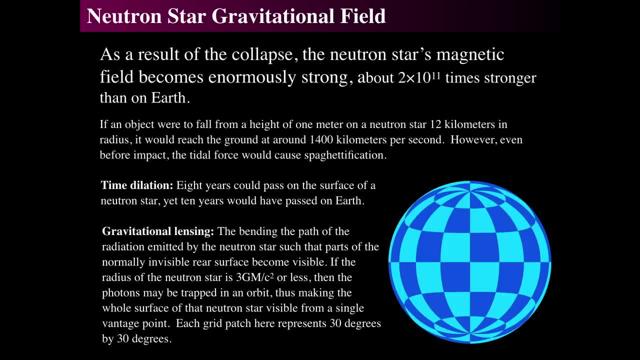 of the earth in the history of the earth. In fact, that would be about the same amount of energy that the sun emits in a few minutes, if not more. I should have calculated that. That's a great calculation, In fact. I will leave that as an exercise for the student, But there's an enormous 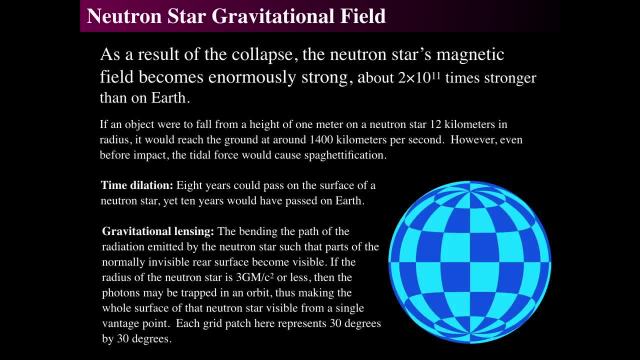 amount of energy that is put there. So we can say an object dropping inside of this will go to 1400 kilometers per second. And if you want to have some fun, you can see the kinetic energy of that by saying: well, what would one kilogram dropped If its kinetic energy is? 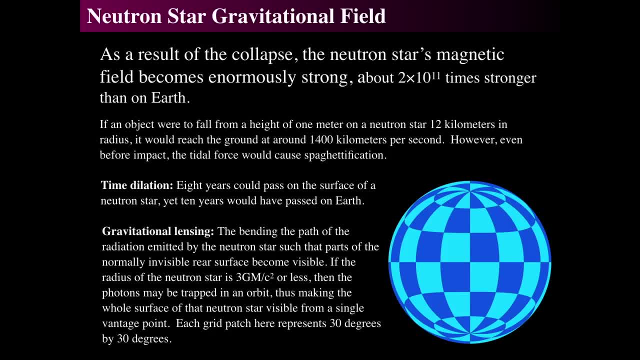 the mass times, the speed squared. what do you get out of that? What's the total amount of energy? And it's an enormous amount of energy that you get, Anyway. so the time dilation, because of general relativity, comes into play. there's actually a time dilation At the surface. 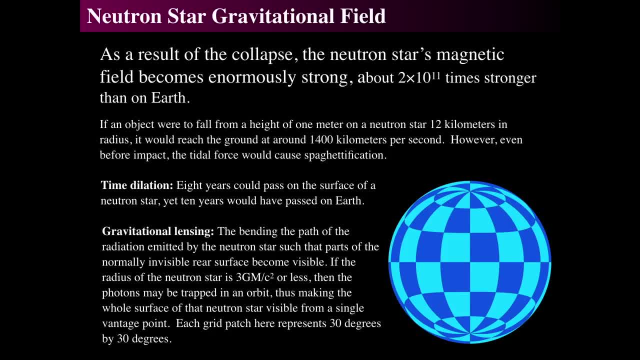 if you had a clock, that clock, if eight years passed on the surface of the neutron star. yet very, very, very, very far away here on earth, where the gravitational field is much less, or even just like a couple of light years away from the neutron star. 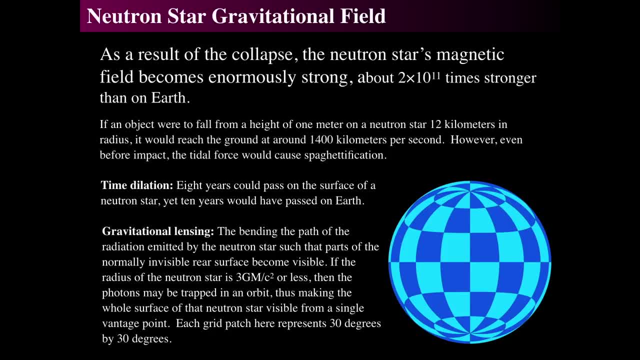 eight years on the surface of the neutron star means 10 years far away from the neutron star, which is very interesting. So there is a time dilation between the surface of the neutron star and far away, So time runs slower on the surface of the neutron star, which is fascinating. 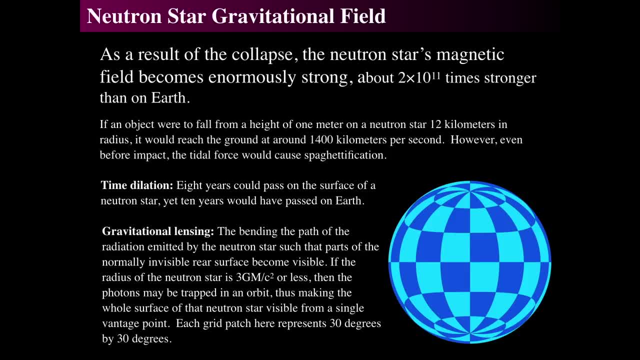 There's also gravitational lensing. that occurs because the path that light takes as it tries to leave the surface of a neutron star, let's say a little gamma ray, gets emitted. It will if it gets emitted at a, at an angle that's not specifically perpendicular to the surface of the 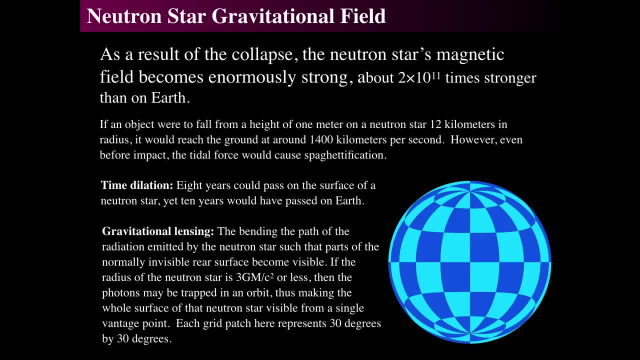 neutron star, it'll start to curve in its path. In fact, what we see in this crazy little image here is what it would look like- Like that if you were at a relatively massive neutron star, you can actually see around the backside of the neutron star. 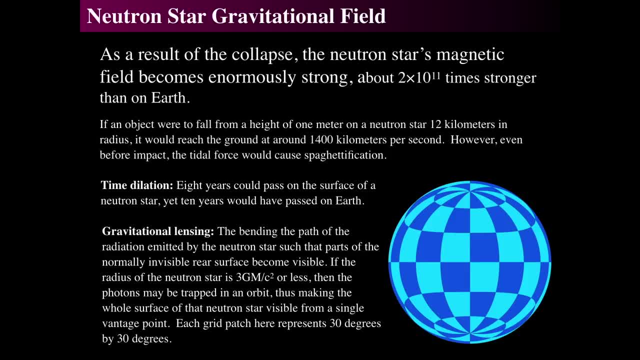 because of the bending of the light due to the gravitational field. So each one of these squared degrees is 30 squared degrees, but you can see that you can see past the poles on both sides, so it looks like you can see more. 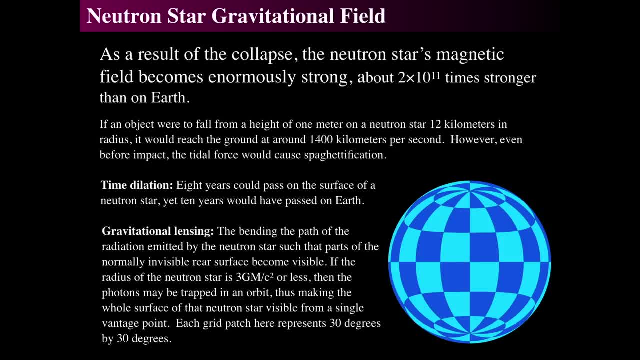 Now, if the radius of the neutron star is small, is actually much smaller because the mass is higher- then you could actually be at a certain place above the neutron star and see the entire neutron star, the front and back, the entire neutron star in your full field of view, because the light could be possibly. 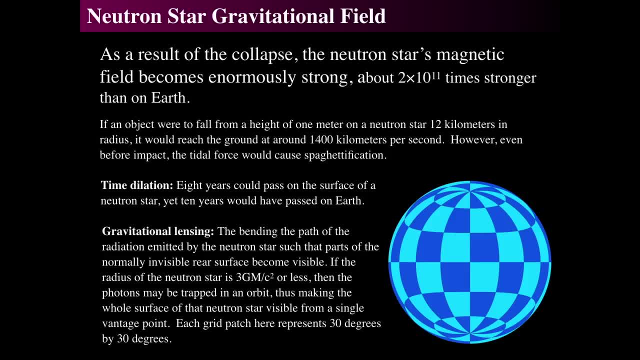 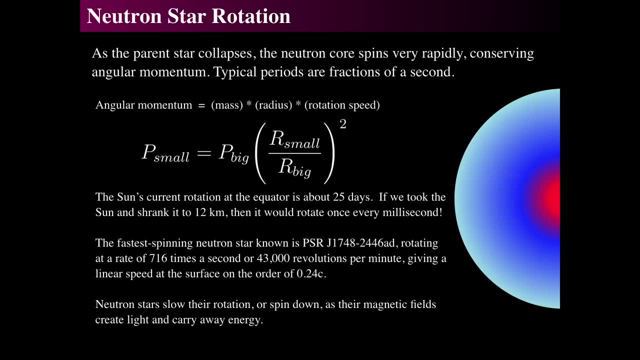 trapped in a circular path around it, And that can happen due to gravitational lensing at a certain radii, meaning the neutron star is going to be very, very massive. All right. so when you take an object like the sun and compress it down, if you took the sun, a whole solar mass- and compressed 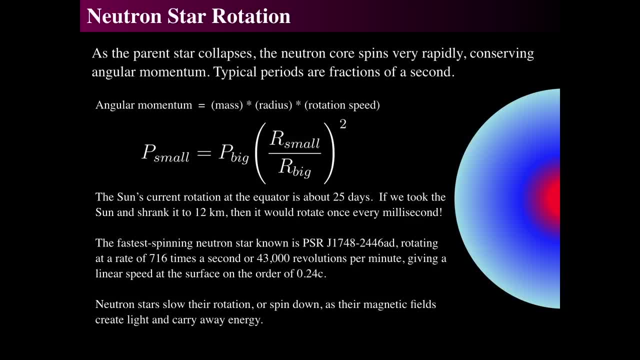 it down to something 10 kilometers in size, then you're going to spin it faster. It will spin faster, and that's called the conservation of angular momentum. So angular momentum does get conserved. and so what is angular momentum? Angular momentum is the product of the mass times, the radius times. 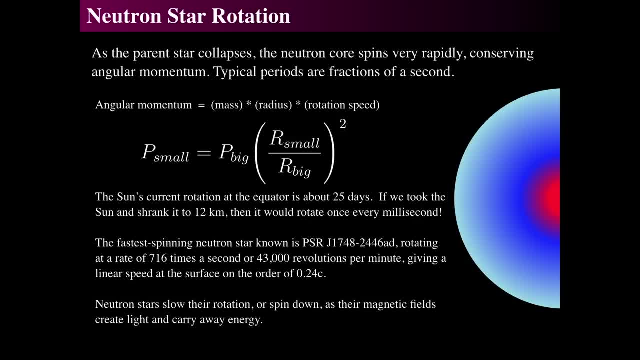 the rotation speed. and that's in very, very, very general terms. So if you keep the mass the same and angular momentum is conserved, because there's nothing keep pushing the angular momentum away, so that is conserved for a given mass, radius and rotation speed. So if that number for the 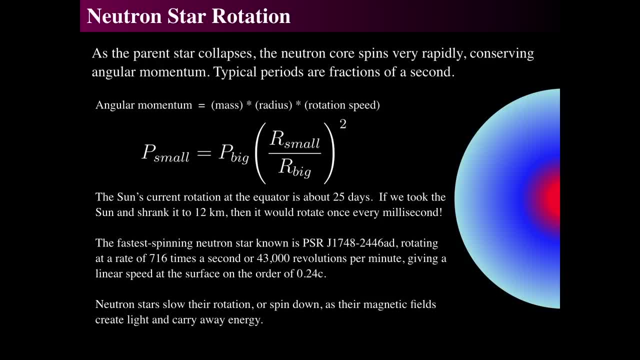 angular momentum stays the same and the mass stays the same and you shrink the radius. therefore the rotation speed has to go way up. So the period of rotation is going to go faster. It'll get faster and faster and faster As it gets smaller and smaller and smaller. So if you took the sun, which is rotating at the equator, 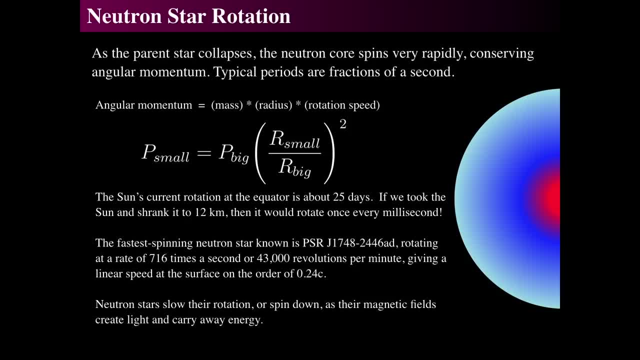 every, say, month or so, and if you shrank it to the size of 12 kilometers it would be spinning about every millisecond or so. And the fastest spinning neutron star is that one with that crazy name and it rotates about 43,000 revolutions per minute, or 716 times a second. That neutron star is. 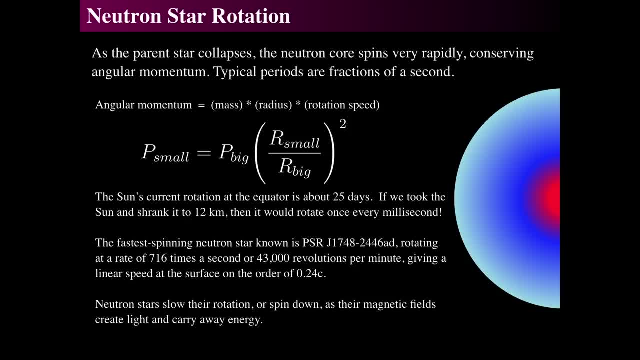 actually spinning faster than a helicopter blade. Helicopters don't spin 700,000 revolutions per second, They spin a few times a second. They do not spin that fast. So neutron stars, things more massive than the sun, spin faster than helicopter blades. In fact the linear speed of that neutron star is about a quarter of. 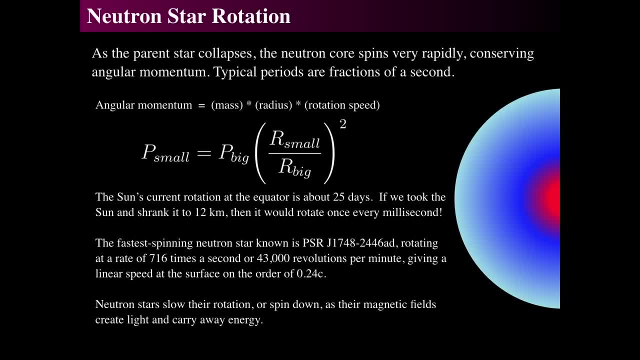 the speed of light. That's how fast it's rotating Now. eventually, neutron stars do slow down or spin down because they have incredibly strong magnetic fields and their magnetic fields interact with the interstellar medium. They also can create light as they spin and that electromagnetic radiation carries away the energy of it and that allows the 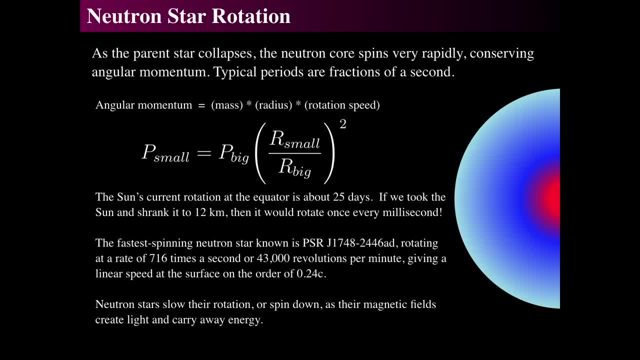 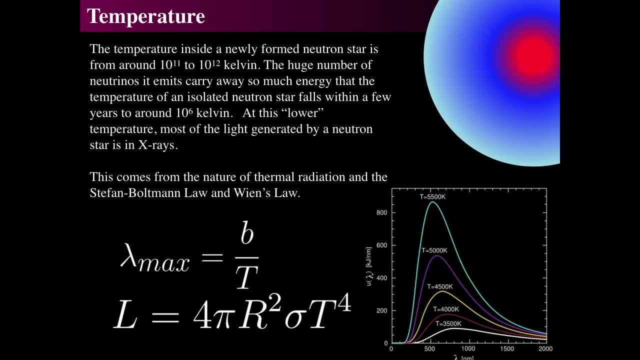 magnetic field to interact with it and therefore carry away the rotational speed or carry away angular momentum by emitting light, which is really interesting. The magnetic field can be so strong it carries away the angular momentum. All right, so now the surface of a neutron star, or even inside. 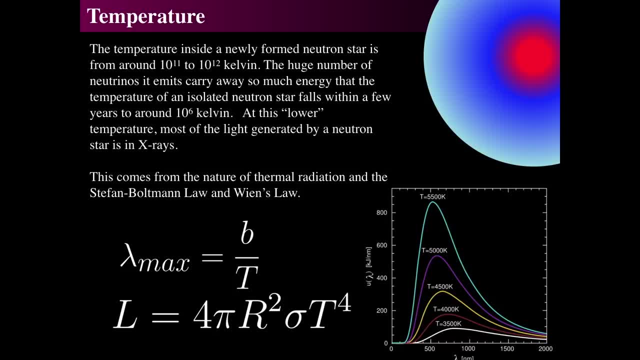 a neutron star is incredibly strong. So if you took the sun, which is a neutron star, and you put it in the center of a neutron star, it's incredibly hot. Remember, they're formed in the forges of super massive explosions of supernovae and so we have when they're formed, they can be formed around almost a. 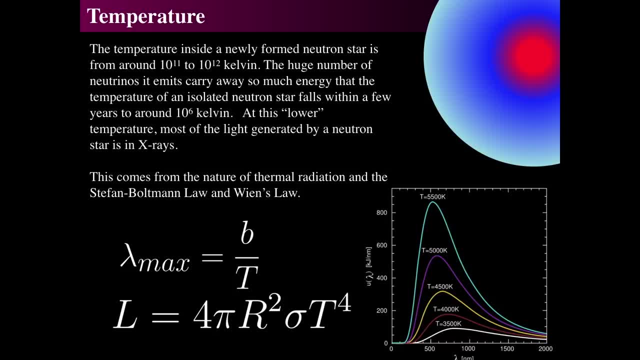 trillion Kelvin, which is just a catastrophically large number. What is that? We can't even put our hands around that. There's no way to really know what that means. However, they keep emitting neutrinos as they do and as they collapse. 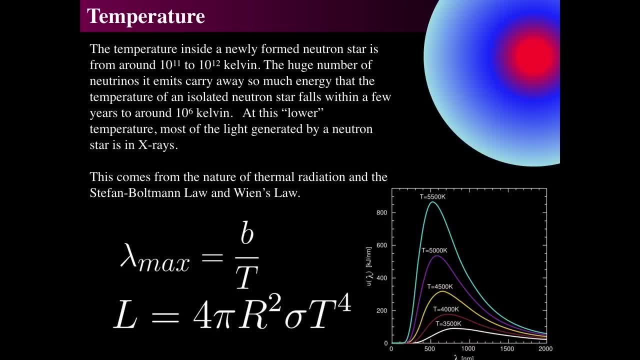 So the neutron star is so hot that the temperature is so high that it actually induces nuclear reactions that carry away energy by neutrinos. So neutron stars fall very, very, very quickly down to only about a million Kelvin, which is still hotter than any other star out there, And what that does is that this lower temperature of a million Kelvin 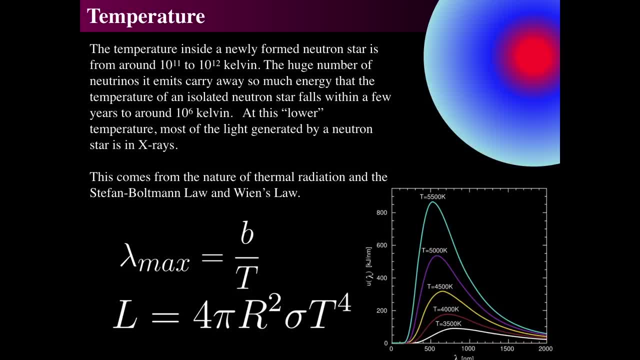 means that their peak wavelength of radiation is way out in the X-rays, And that is if we have a neutron star. we know, if we assume that the neutron star is at the same temperature and that it is thermalized, meaning it has a black 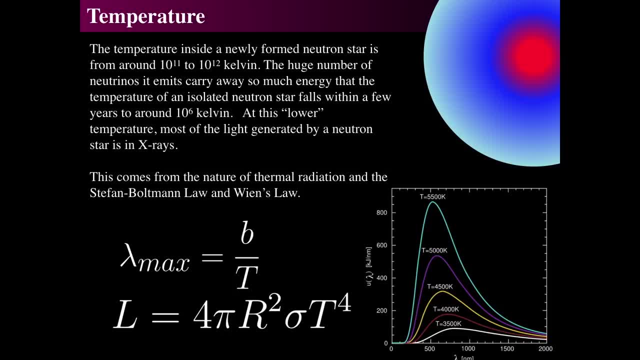 body spectrum, then we can use the lambda max equals B over T thing that we learned way back, which is Wien's law and the Stepin-Voltsman law, to determine the luminosity of it, given the radius, And we find, if we know the peak wavelength out in 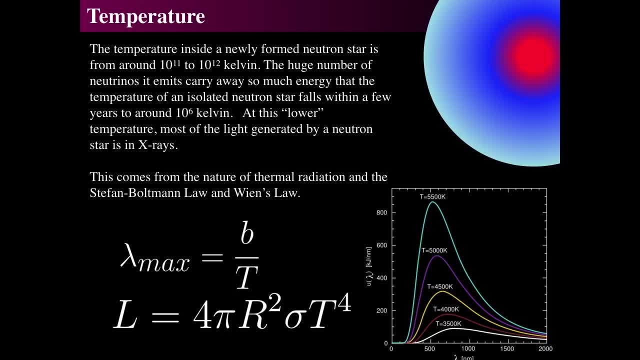 X-rays. that gives us a very, very, very high temperature, But the radius is insanely small, So that means the luminosity is really tiny. So these things that we have to be careful about, The luminosity of the radii is really tiny. It's like it's a very, very small minus. And for me 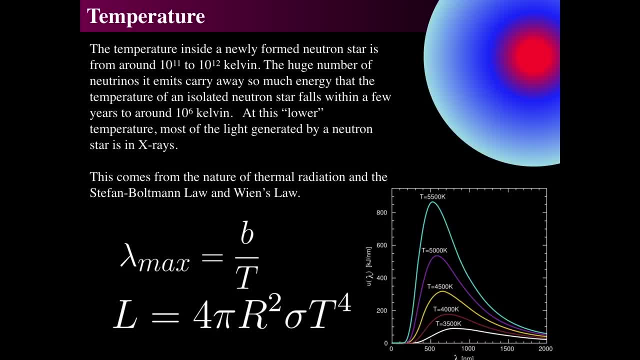 These things even though the luminosity should be incredibly bright because of the temperature, the radius more than undoes the effect of that. So the luminosity of these things is very, very, very small. And just to give you an idea, that inset is a graph of you know. 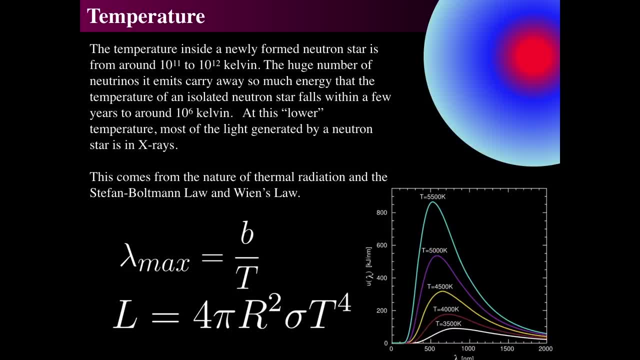 some typical cool stars that are between 3,000 and 6,000 Kelvin. The emission from X-rays would be really huge because they would be in millions of Kelvin, which would make these graphs look like little tiny bumps, And these would look like a tiny bump next to a mountain. 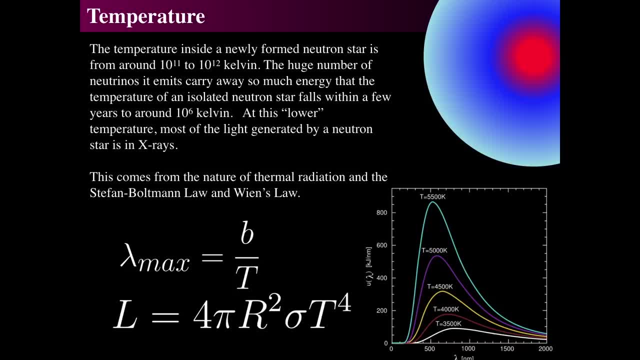 which would be how big these bumps would be. But that would be over a small amount of surface area, And the surface area is really small, So the luminosity is tiny, So the temperatures are really hot. Now here's a really cool thing. 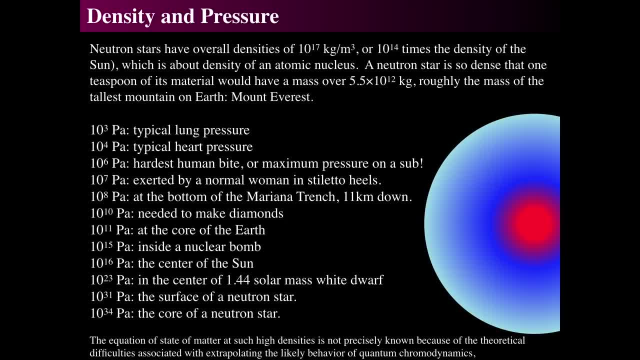 When you take something and you make it really small, you have this huge amount of mass and you compress it into a very small volume. you raise its density, And so the densities of neutron stars are really big, like 10 to the 17th kilograms per square meter. 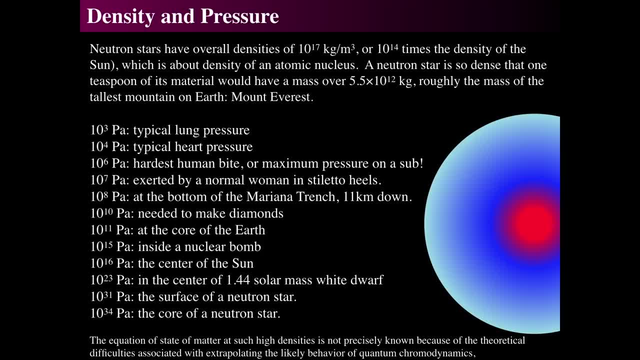 which is about the, which is almost, which is: it's just. that's insane. It's 100,000 times, 100,000 billion times, the density of the center of the sun. Okay, that's what 10 to the 14th times the density of the sun means. 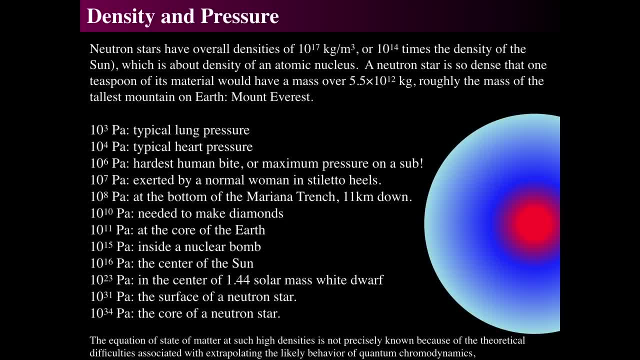 The sun is. it's more than 100,000 billion times the density in the center of the sun. Isn't that wild That is? that's just out of control. which is the same density as an atomic nucleus, roughly speaking. 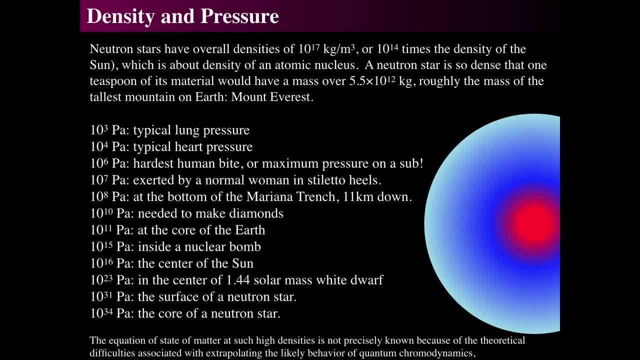 So a neutron star is so dense that one teaspoon, which is about the same size as a cube of sugar, would have a mass of the tallest mountain on earth, all of Mount Everest, all in one place. So take Mount Everest, compress it down. 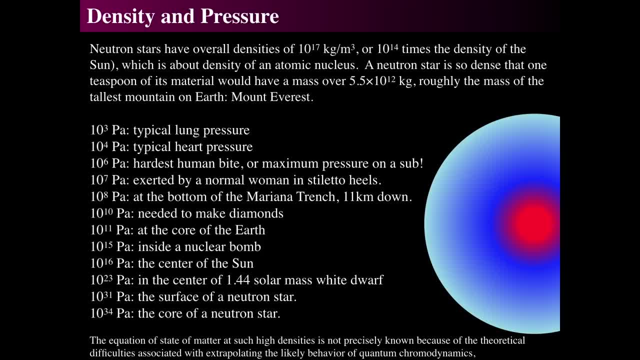 to something half the size of a cube of sugar and you've got the density of a neutron star. Now that means the pressures are incredibly, incredibly high. So, oh, just one last thing about the density: If you go and look at Marvel Comics, 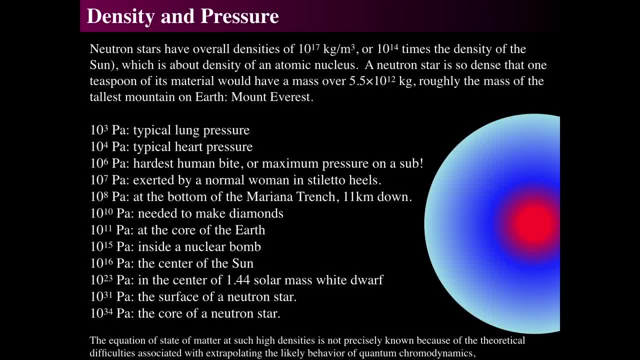 shows the character Thor. Thor, the God of Thunder, has a. his hammer is mounted on a neutron star. Yeah, that'd be pretty tough to lift unless you were a god. So luckily Thor is a god, so he can lift a neutron star. 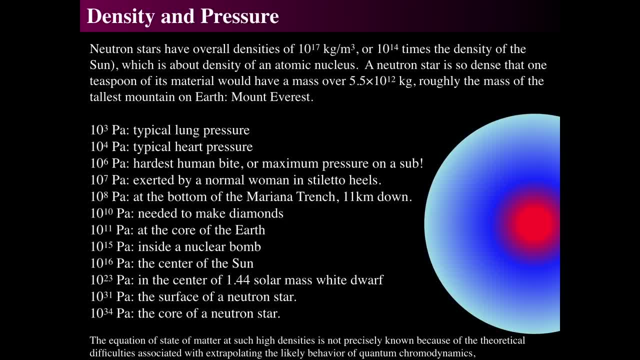 But by rights nothing else can lift it And somehow something with that density somehow doesn't do anything. when he sets it on a table or puts it on somebody, Yeah, it should have such an incredible gravitational interaction that it pretty much destroys everything around it. 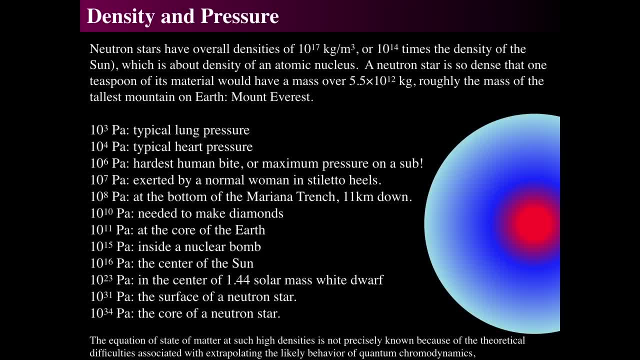 So somehow it can't be lifted by anybody, but yet he can set it down on a table or on the floor of a building. It's really kind of weird. It's just. you know, how can you set it down on anything? 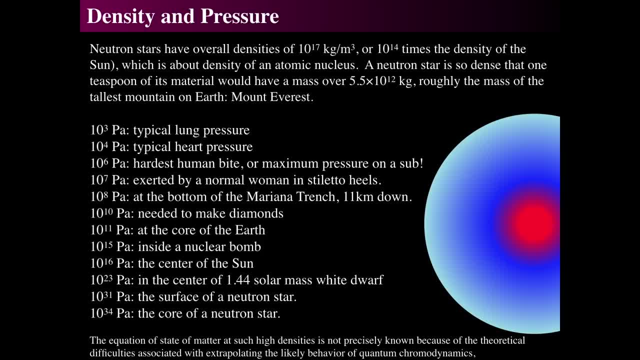 and have it not go right to the center of that thing. Well, hey, it's comics. What can you say? All right, but that's kind of fun to think. In any event, we can then look at the pressures that happen. 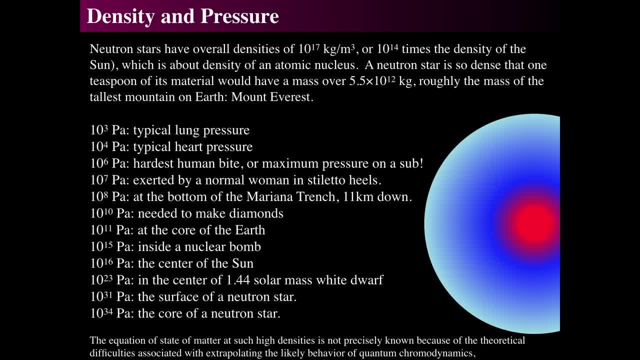 And I saw I found a really cool list of pressures. So it's fun to think that 1,000 pascals, where a pascal is a measurement of pressure. So your lung pressure when you breathe is about 1,000 pascal. 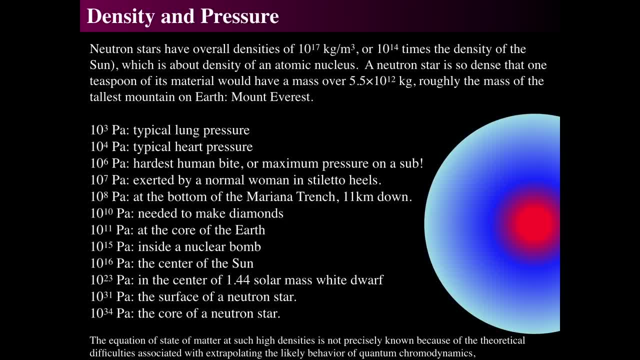 About 10 times that is heart pressure. About a million pascals or 1,000 times your lung pressure is about as hard as you can bite. Or more specifically, if you put a zillion people biting on a nuclear submarine. 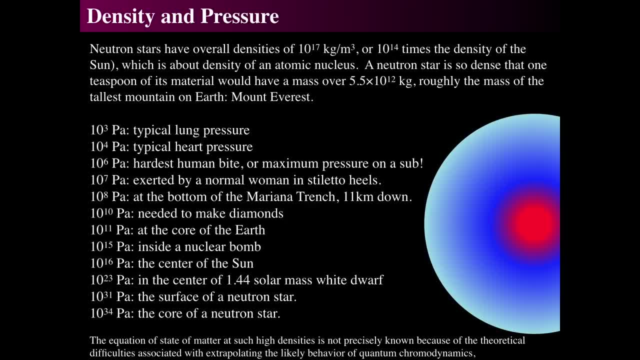 that's about this pressure that the nuclear submarines hull can take, And that's the same as a nuclear class submarine can take if it goes down about 500 meters. That's about a million pascal. Funny, though, is that you can also then take lots of women. 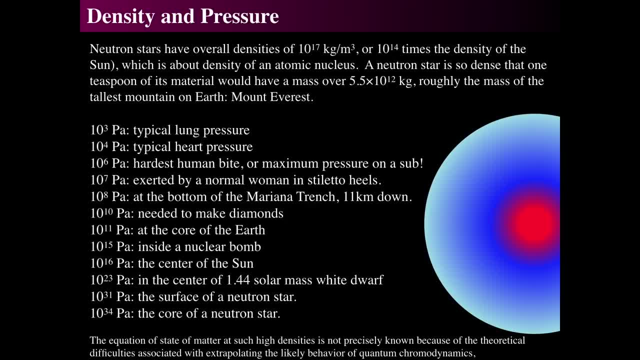 in stiletto heels and have them all walk on the surface of the submarine. Now, if all these stiletto heels where women were walking, such that they all stomped with their stiletto heels so there was no free space on the surface of a submarine. 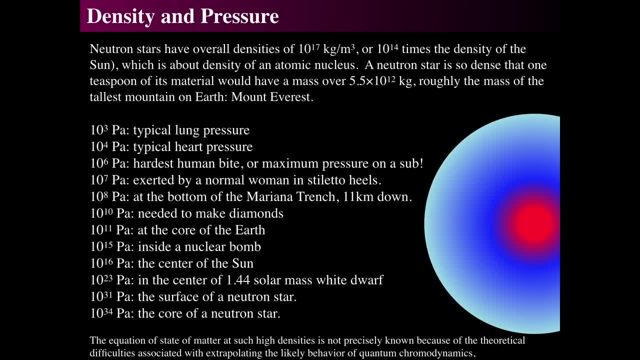 they would crush the submarine, Because a normal woman in stiletto heels is 10 million pascals. So if many women- so that all their heels were linked together so there was no space between them- all hit the sides of a submarine at once. 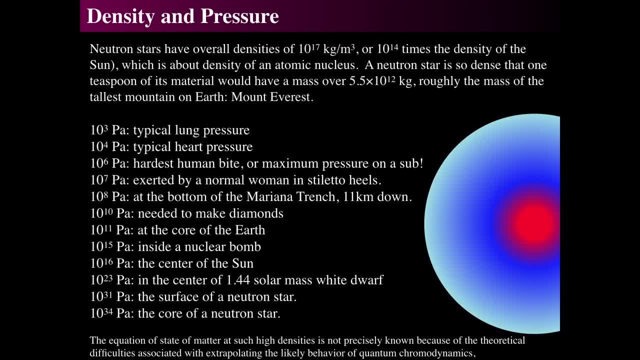 they would crush it. Interesting Power to stiletto heels. So 100 million pascals is the bottom of the Marianas Trench, So really that's a huge amount of pressure. 10 billion pascals need to make diamonds only a thousand times more. 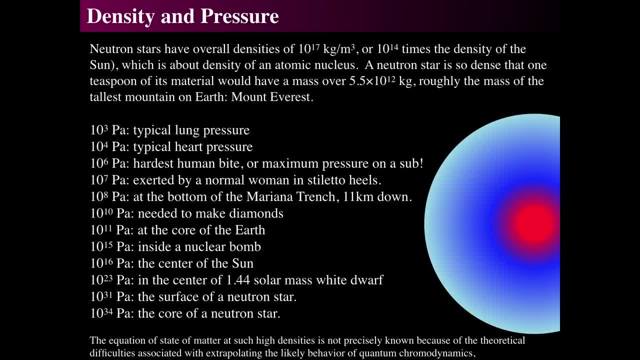 than what is made by women walking in stiletto heels Fascinating. The pressure of a nuclear bomb is 10 to the 15th pascal, which is 10,000 times what it is at the center of the Earth. 10 times greater than a nuclear bomb is what's at the center of the Sun. 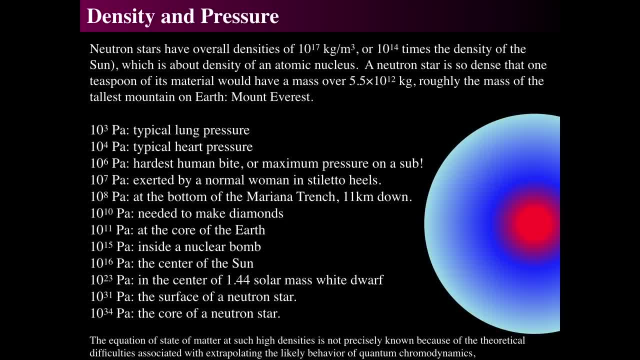 Well, now we're getting up to insane numbers. 10 to the 23rd pascal is the center of a Chandrasekhar-limit solar mass white dwarf, A Chandrasekhar mass white dwarf. 10 to the 31st is the surface of the neutron star. 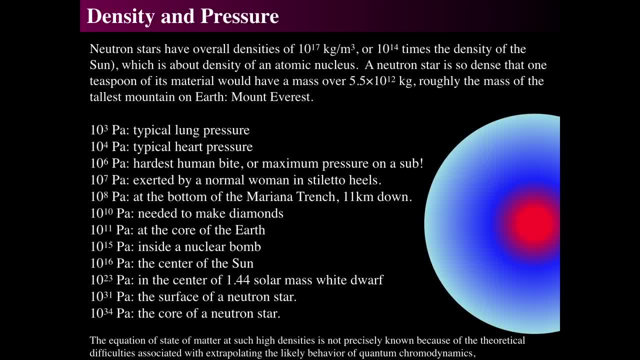 and 10 to the 34th pascals is the core of a neutron star. There's just really nothing to think about these things. It's just very strange. So because remember that the equation of state for materials links density, pressure and temperature. 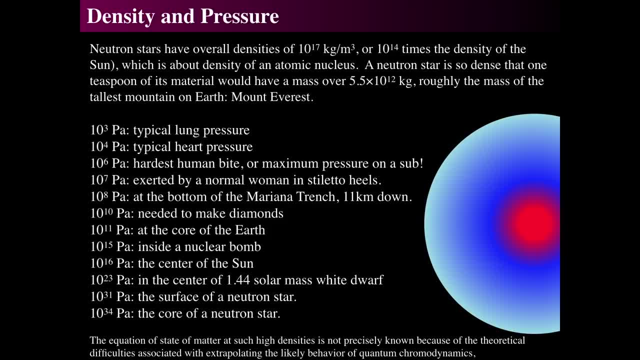 under these incredible, incredible conditions, there's no way to really get the. there's no really good state of matter at these densities, So it's all very theoretical and you have to take into account quantum chromodynamics, general relativity, many and 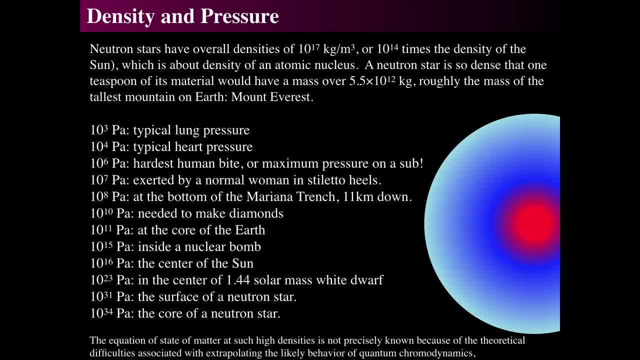 lots of things in order to actually understand what's going on. the strong nuclear force and it just is a real mess to try to understand what's happening down there. So the equation of state and exactly how they go is not well known. We don't have it like we have in the previous lecture for white dwarfs. 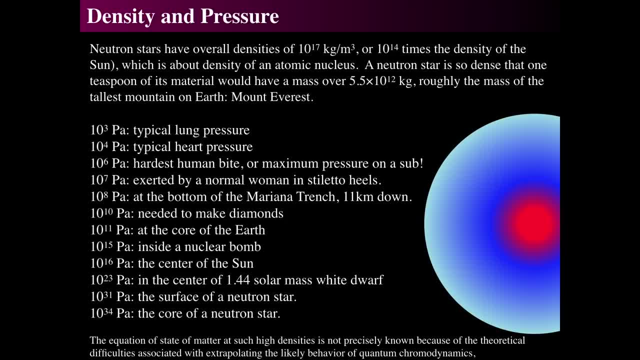 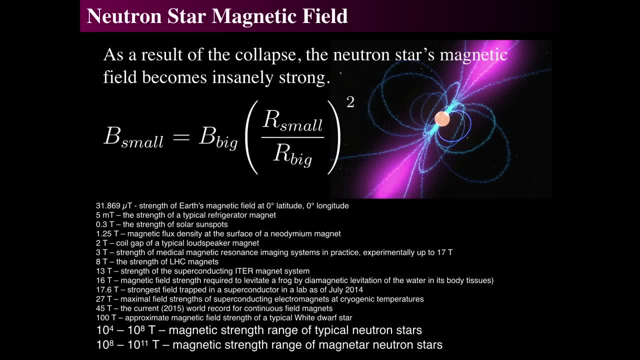 approaching this Chandrasekhar limit. All right. So the other thing is is that we talked initially about the Sun with its magnetic field. Likewise, stars have magnetic fields, So there should be a magnetic field, And so the magnetic field becomes wildly strong as the neutron star collapses. 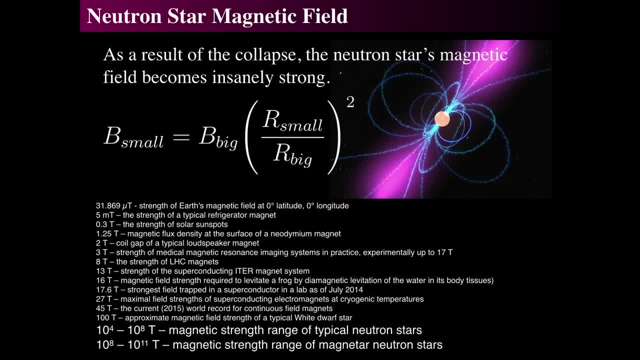 So it's hard to know what magnetic field kind of strengths are. But the fun thing is we can say the 31 micro, 32 microtesla. So the Tesla is a unit of magnetic field and it's the SI unit of magnetic field. 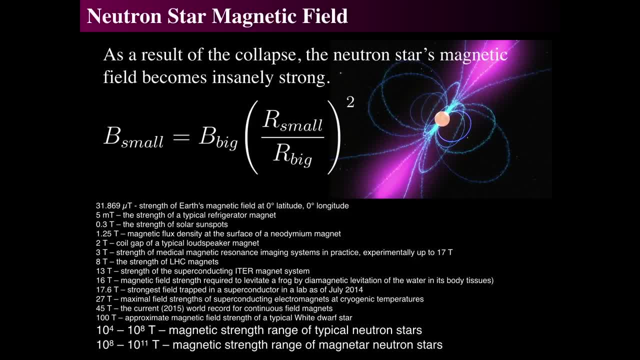 So 32 microtesla is the strength of the Earth's magnetic field. So if you pull out a compass and just say what's north, that's what is. that's why you have to have a very, very balanced thing, because it can get messed up by other magnetic fields around you. 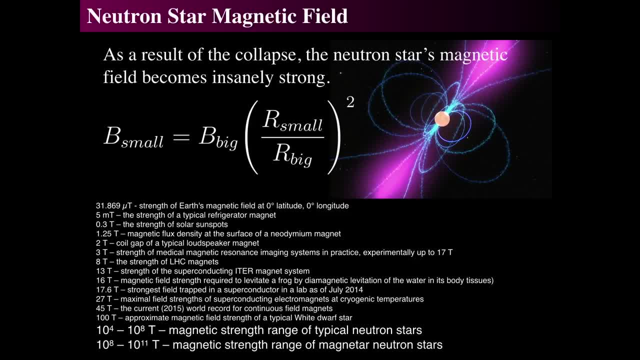 And if you bring a refrigerator magnet next to it which is 5 millitesla, which is, you know, 100 times strong, stronger than the Earth's magnetic field, then a typical compass will point at it. So that's 5 millitesla. 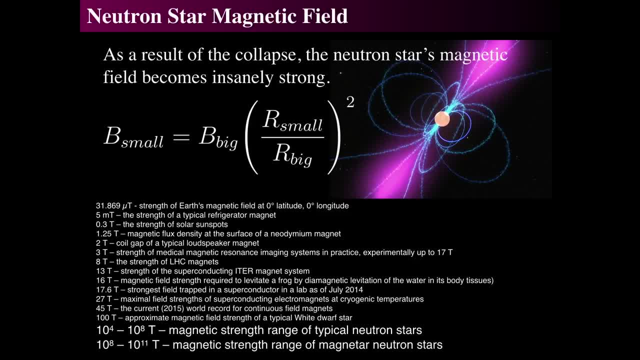 And the solar, the sunspots on the surface of the Sun, are about about three tenths of a Tesla, And those things actually serve to show you the Zeeman effect, which actually can be measured. So that's actually a pretty strong magnetic field. 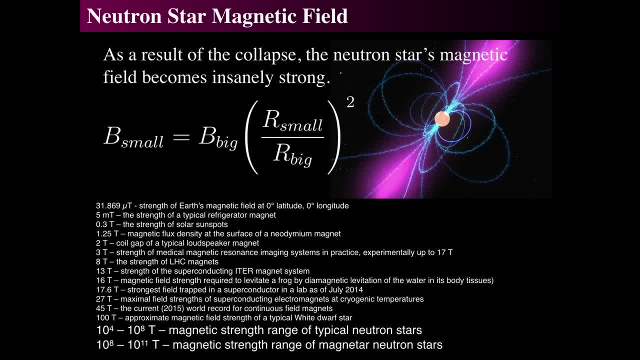 is three tenths of a Tesla, Then the very strong Tesla, like one and a quarter Tesla, is what you have with very strong magnets that you can buy, say, off of Amazon one and a quarter, And if you go and buy, if you go take apart a loudspeaker. 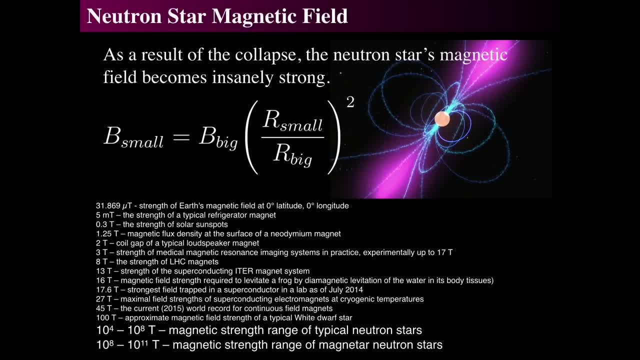 like some big loudspeaker, like a big audio loudspeaker, and then look at the coil gap that they have inside of it. inside the gap that's even stronger. Again, it's about two Tesla If you go get magneto MRI at a lab. 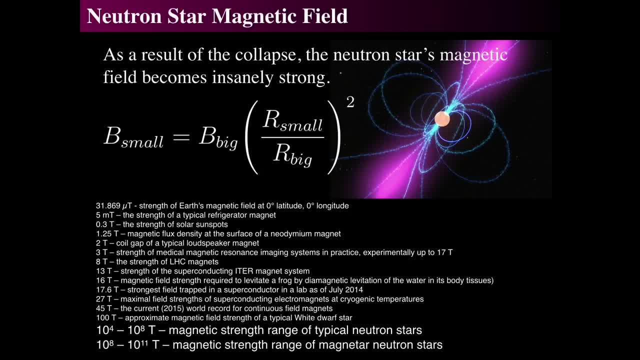 you're going to be experiencing about a three Tesla thing, and some of those can go up to 17 Tesla. The Large Hadron Collider has magnets that are about eight Tesla and those things serve to confine extraordinarily hot plasmas and they can bend. they can bend the paths of protons and electrons. 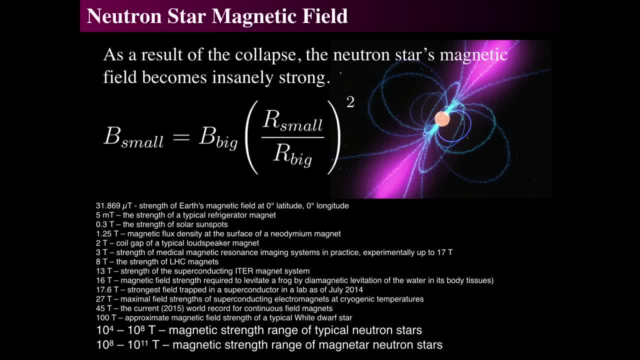 going at nearly the speed of light. That's what eight Tesla can do, And they're some of the strongest magnets known. But the ITER experiment, which its goal is to try to instantiate nuclear fusion, and that's what the superconducting magnet system is for ITER. 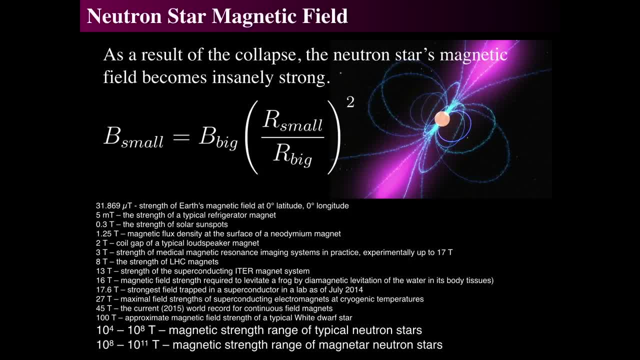 those are only 13 Tesla. 16 is kind of a funny thing. There's some really funny videos about you can levitate a frog with 16 Tesla and the water molecules will actually align and then go against the, the magnetic field. 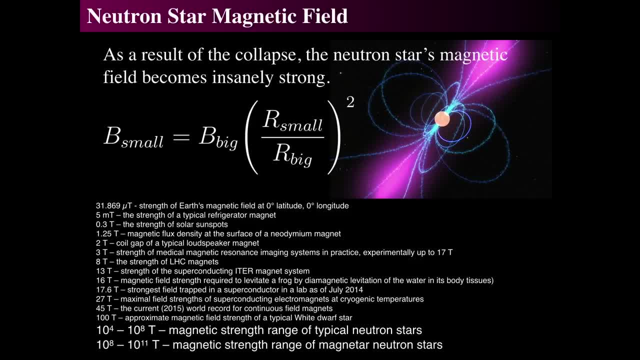 and that makes the frog float. So have some fun. Google floating magnetic frog and you'll see some funny videos. A little bit stronger than that is the, our experimental magnetic resonance imaging, which is the strongest magnet, which is the strongest superconductor in the lab. 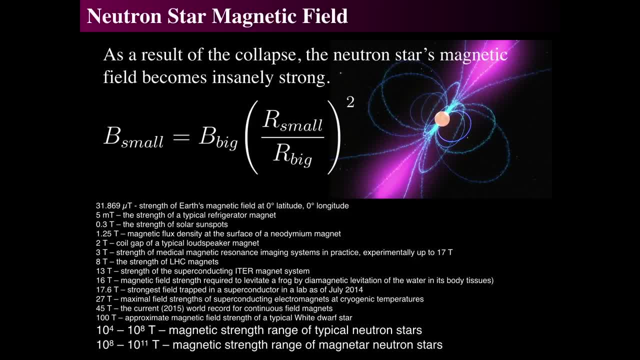 And the maximum strength for short period magnets is about 27, and 45 is continuous. 100 is the surface of a newt of a white dwarf, But neutron stars have 10,000 to 100 million Tesla. There is literally nothing else out there that does this thing. 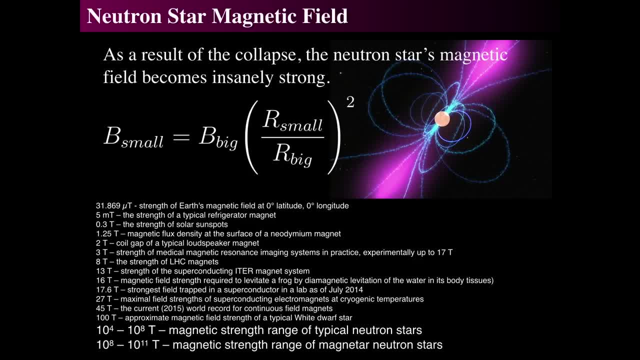 that the sun can't do it, white dwarfs can't do it, nothing can do this except neutron stars And magnetars, which are supremely magnetic. neutron stars are between 100 million and 10 billion Tesla. Now, if we then say: 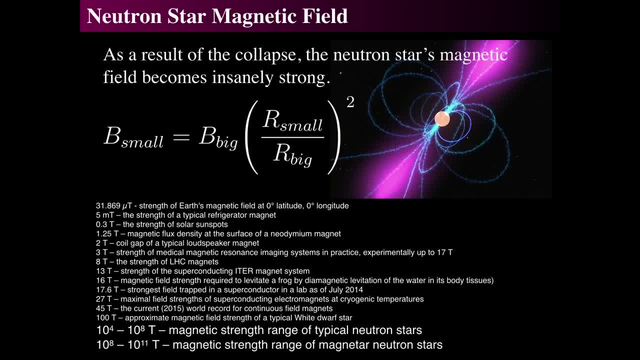 well, how big is this magnetic field? If we took a magnetar at the top end of that range, which is, say, 100 billion Tesla, and that neutron star passed within the orbit of Pluto, that would demagnetize every hard drive on Earth. 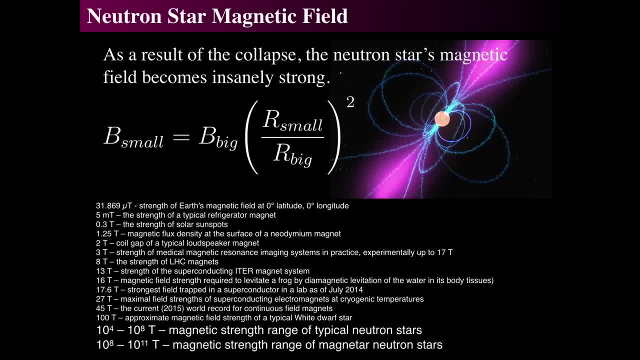 at 40 astronomical units, That would be a bad day. So yeah, these things are insane- insane magnets, So they would have visible effects on the solar system. at one light year away, A magnetar would. So if they got really close, it would be bad. 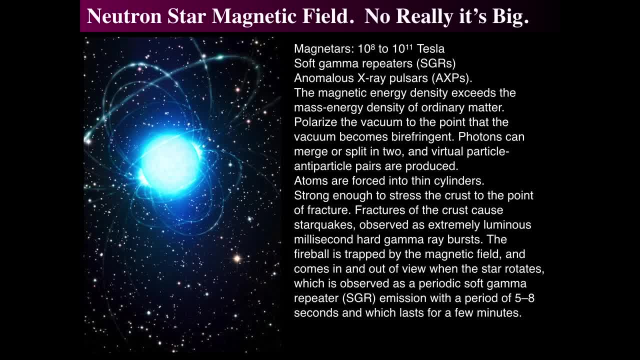 So let's look at those things. These things are really, really, really bad. So let's say, the magnetars are incredibly strong and they are possibly the sources of particular gamma-ray bursts, called soft gamma-ray repeaters or anomalous X-ray pulsars. 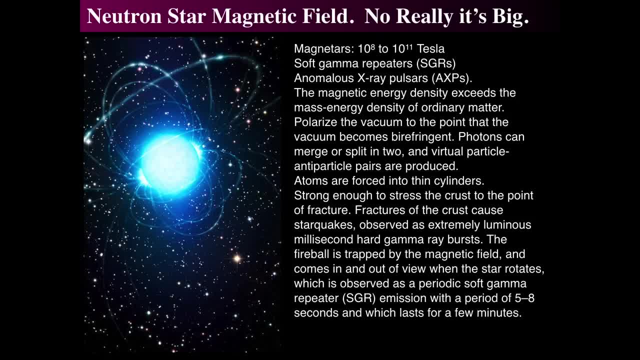 So what's happening with these magnetic fields that become that strong? The magnetic fields can be so incredibly strong that the energy density inside the magnetic field is larger than is required of ordinary matter. So we can say what is E equals mc squared for a proton. 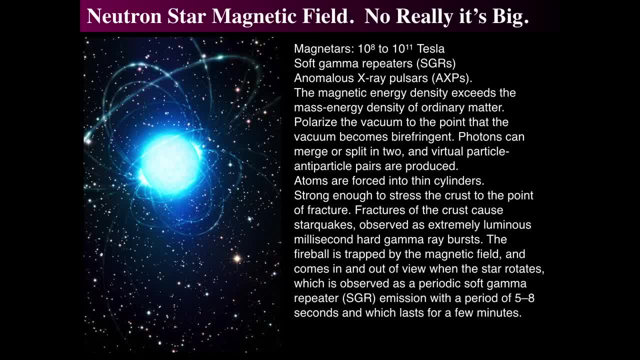 What is E equals mc squared for an electron, And the magnetic field itself in space exceeds that of the energy of an electron and proton in mass. And what it can do is that the magnetic field can polarize the vacuum, In fact the vacuum of space itself. 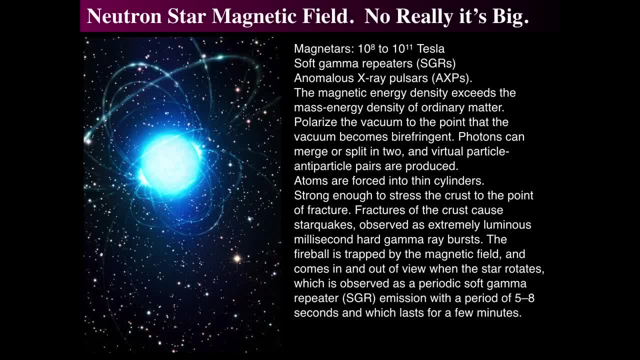 then becomes polarized by the magnetic field and the space itself becomes what's called birefringent, And birefringent means that space itself has multiple ways that it can refract light. So go back and look at our refraction. 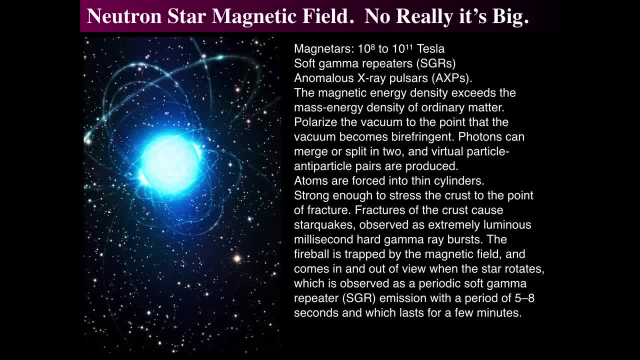 We think of a refracting telescope. It refracts the light, It changes the direction. So when it's birefringent, it depends on the polarization of the light and depending on the polarization of the light, a photon can be split apart. 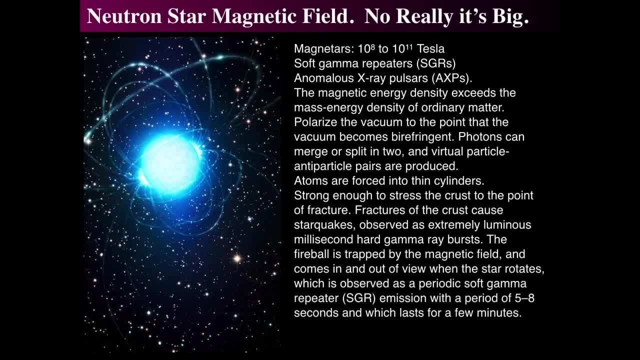 and the light can be split or split apart or forced to merge. And if photons can be forced to merge, then they can create particle-antiparticle pairs, such as protons and antiprotons or electrons and antielectrons, which is really crazy. 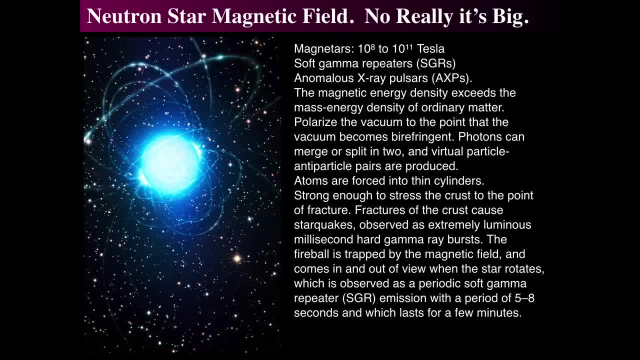 Once those things are created, then those proton-antiparticle pairs and antiproton pairs can then recollide and form gamma rays Also. such strong magnetic fields take atoms and they force the atoms to become, instead of spheres, the atomic radii, become cylinders or needles. 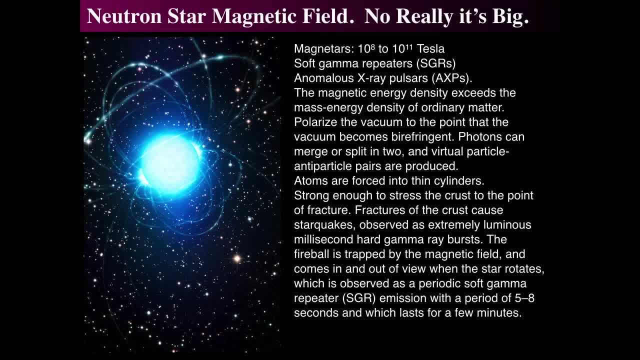 So atoms as they exist around us cannot exist because we think of atoms as having that nice little Bohr radius, where it's like electrons are zipping around in spherical distributions or radial distributions. No, They become cylinders, which is very, very, very strange. 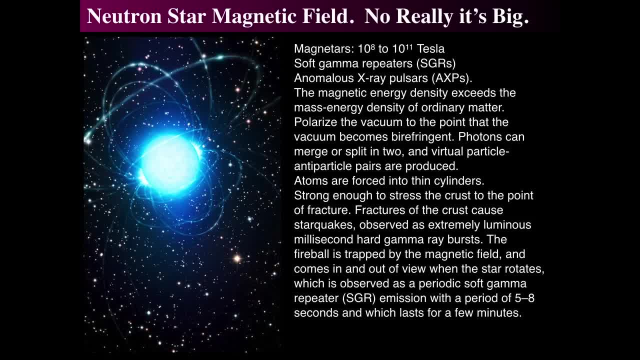 So atoms can't exist, or chemistry that we know it can't exist near neutron stars. So molecules themselves melt close to neutron stars because of the reshaping of atomic structure. So that means that the magnetic fields themselves become so very strong that they actually stress. 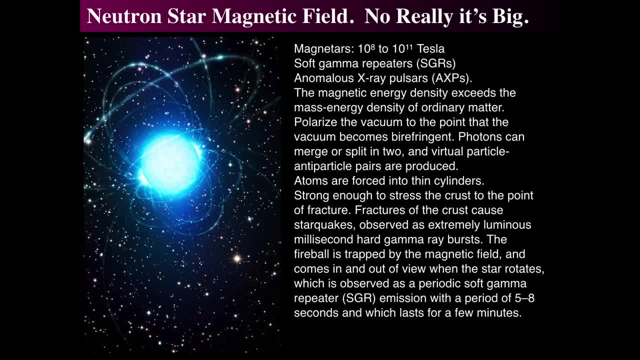 the crust of a neutron star and fracture it. So, remember, the density is incredibly high, but that's enough to actually push the nuclei apart, because they're being deformed and they stress and fracture them. That makes a starquake, which then emits huge amounts of gamma rays. 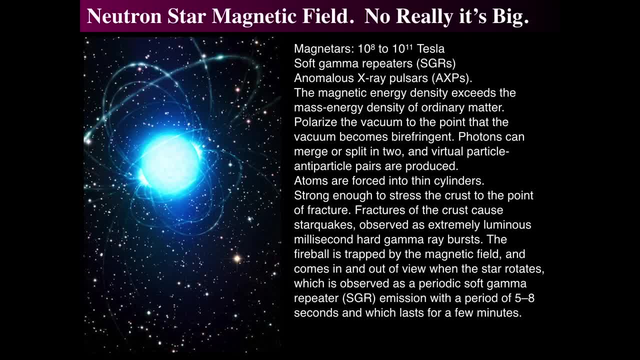 Those gamma rays then make a fireball which then get trapped by the magnetic field And that trapped magnetic field, then the light becomes trapped and as the star rotates becomes a bursting, a burst of gamma ray burst or a millisecond gamma ray burst. 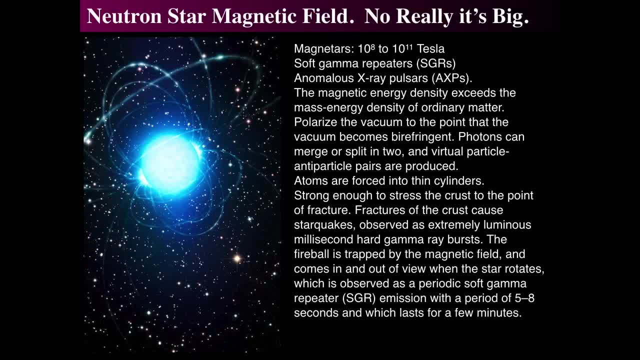 So you get these whips of things that you have, of a series of gamma ray bursts that go bip, bip, bip, bip, bip, many times in milliseconds, So as it comes in and out of view, as it rotates, So these things last only a few seconds. 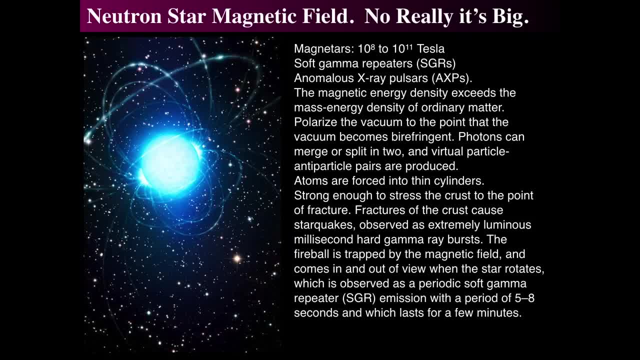 and have been observed by the Fermi Gamma Ray Telescope, as well as the Swift Observatory as well. So magnetars are the most powerful magnetic field in the cosmos. So once again we talked about the equation of state and, like we said before, you don't get. 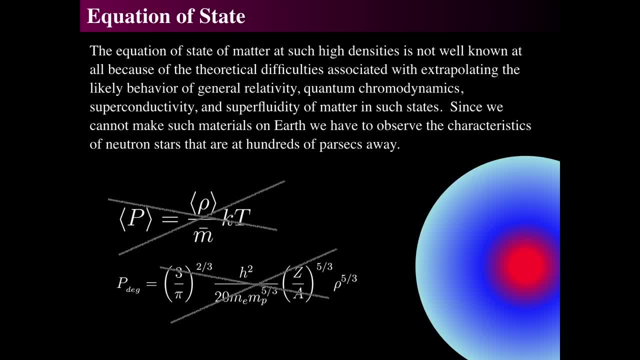 it's just like we have before. we have the ideal gas law which relates the pressure, density and temperature. No, that's not. you can't have that on your neutron star. And what about the relativistic electron degeneracy pressure? Nope, you don't get that either. There's something else going on inside of neutron stars. In fact, the study of neutron stars and their equation of state is an active area of research, And nobody really knows exactly what the equation of state is. 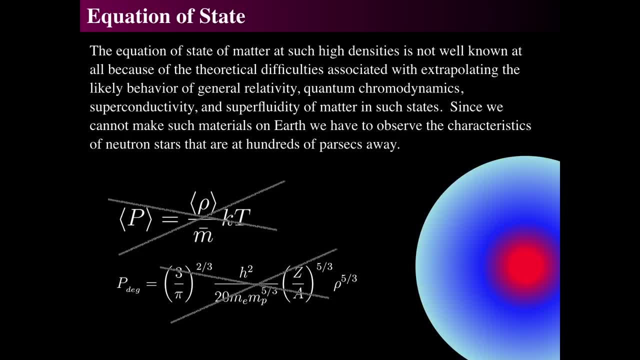 because you have to take into account many, many things such as general relativity, quantum thermodynamics, superconductivity, superfluidity of matter, And it's very. you can't even make these materials on Earth. I mean, it's impossible. 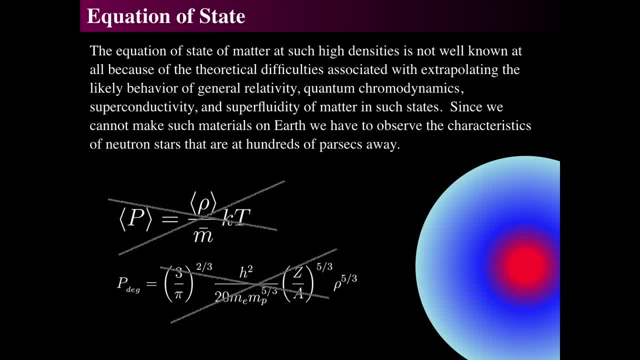 So the only way to observe them is by finding things. but those things are hundreds of parsecs or thousands of parsecs away. So the the equation of state is strongly dependent upon the size and temp and observed temperature of a neutron star and rotation rate. 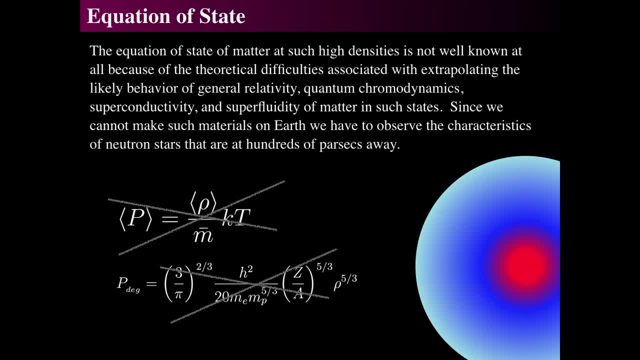 So one of the important things that that astronomers can do to understand neutron stars is simply find the radius of a neutron star, And there's not many that are close, but there is one that is very close, that's relatively close that people keep trying to study in order to get it. 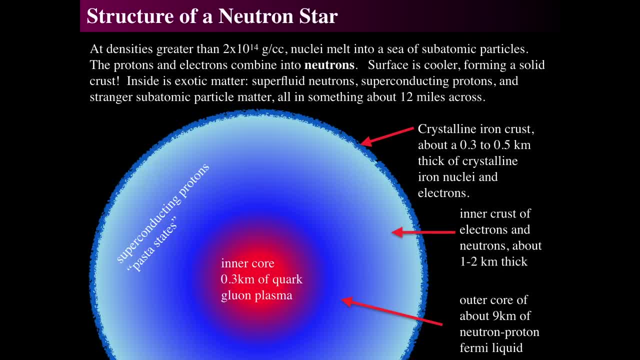 And we'll get to that soon. So the structure of a neutron star inside. remember we talked about the sun. it has a core structure and so forth, But the structure of a neutron star is really fascinating because this thing's only a couple miles. 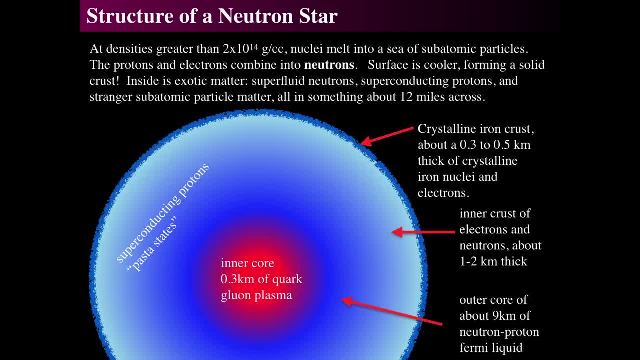 you know it's only 10 miles across. So what does it kind of do? Well, with these incredible densities, we get this very strange crust, And the crust it's a solid. This thing is a star, that is a solid. 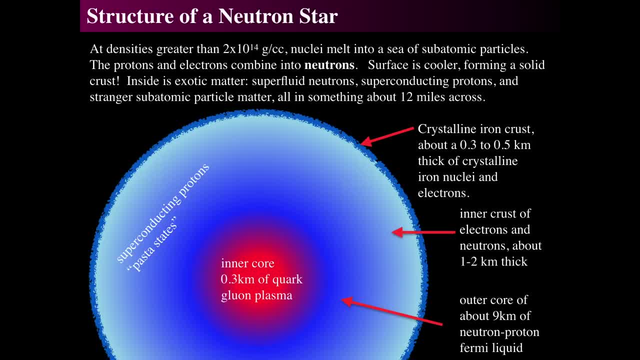 And the surface is basically an iron nickel solid at the crust, which is about um just a half a kilometer thick, And it is a thick crystalline iron nucleus crust with electrons that go around. So you have just basically a hot ionized gas. 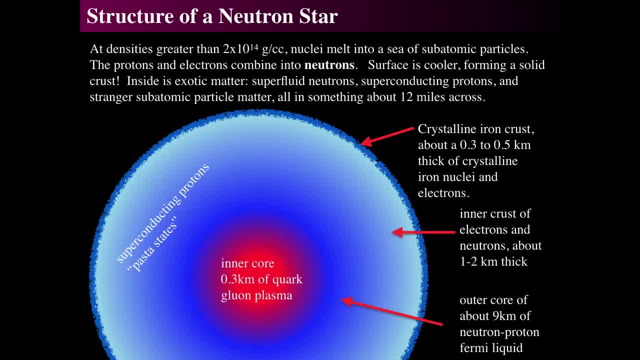 of a million Kelvin And it's a hot ionized gas. that's a solid which is really weird to think. Is it a gas? Is it a crust? What is it? It's kind of a weird thing. Inside of there is an inner crust of electrons and neutrons. 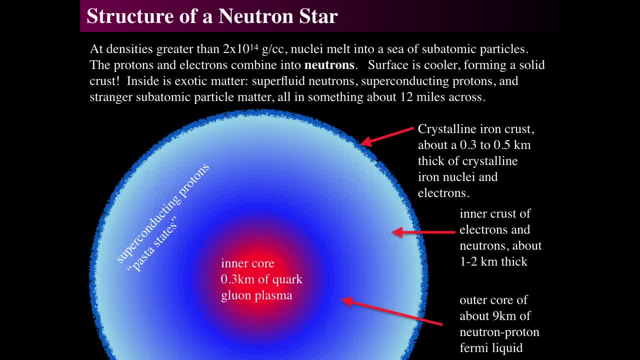 about a kilometer or so thick, And then there's an outer core and an inner weird core, And there should be these weird superconducting states. But recently- in 2017, there was a fascinating study that actually kind of got at. 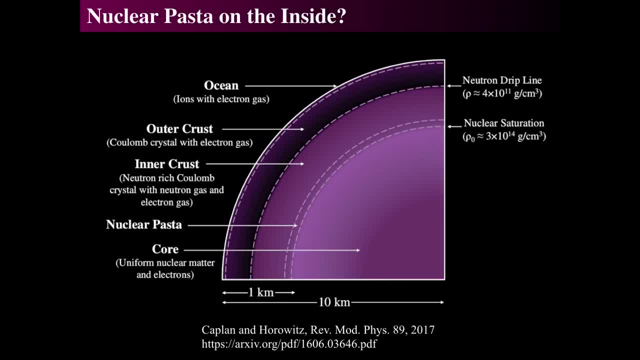 what these states can really look like. So the surface of the neutron star is an ocean of ions or a crystalline crust. The ocean would be an electron gas with a crust of of of ions across it, And then the outer crust would be. 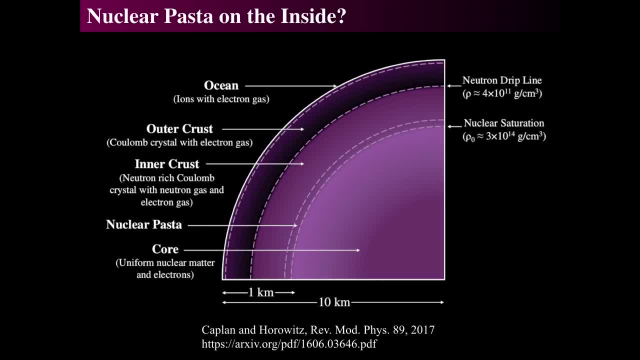 a crystal of, of, of, of, of iron and silicon nuclei with an electron gas. Remember, the electrons stay a gas, but where the nuclei would be would be thick And then the inner crust would be more neutron rich, And then you get this weird phase called. 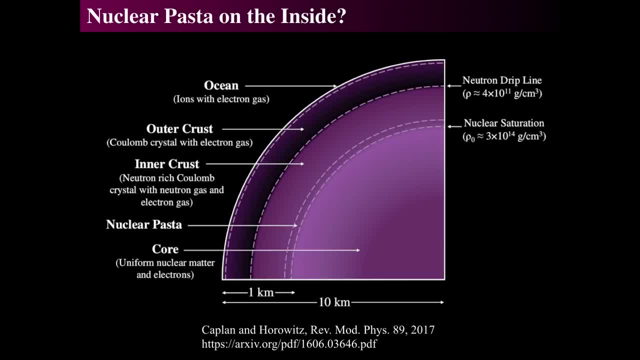 nuclear pasta And it's not some flying spaghetti monster thing. We'll talk about that in a second. But inside, between the crust, where there's actually nuclei, inside of the core there are no longer any nuclei, It's just so dense. 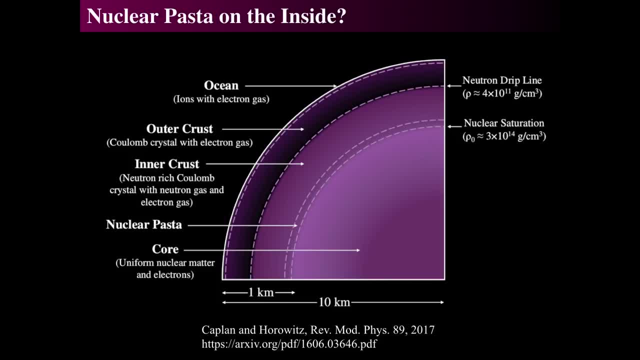 It's just so dense that nuclei don't even exist And you just simply have one big nucleus. So the inner nine kilometers is essentially a uniform nuclear matter where it's just a sea of touching protons and neutrons- mostly neutrons and electrons. 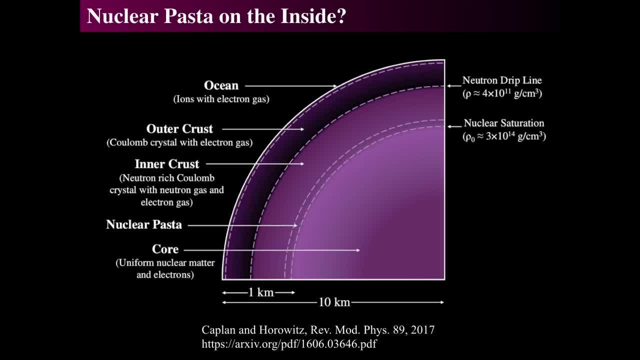 So that's what's interesting. But what do we mean by this nuclear pasta thing? And this was a study done by Kaplan and Horowitz. It was shown in the Review of Modern Physics in 2007.. And there's the link in the archive before. 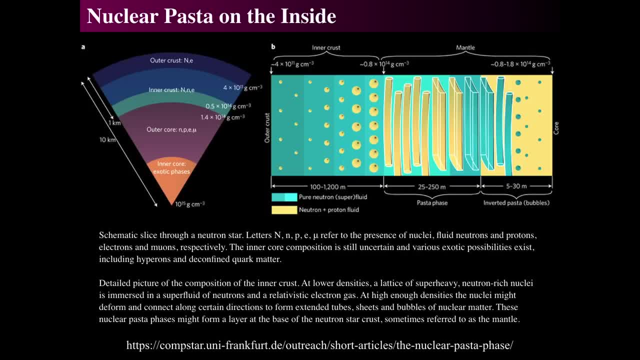 But I'll get to it a little bit more. So what happens is is that there's a slice through it, And so the outer crust is neutrons and electrons, And the inner crust is nuclei and electrons, And then the inner crust is neutrons. 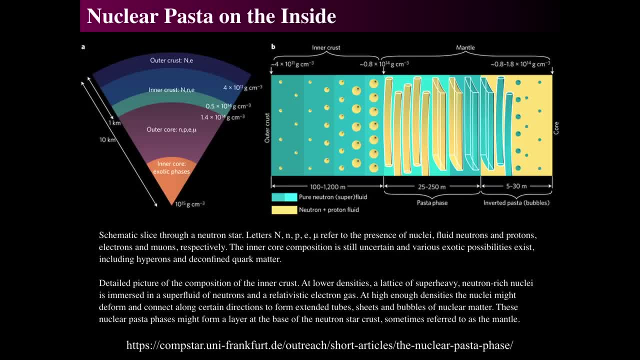 electrons and nuclei And then the outer core. you don't have any nuclei anymore, It's just neutrons, protons, electrons and muons. And then you have weird stuff, exotic phases, in the inner core. But there's a very strange thing that happens. 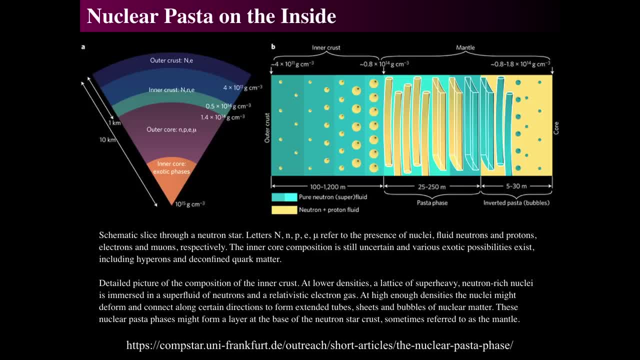 in the green middle region- Right in there It's called nuclear pasta- And where it actually goes to this very, very strange phase Where you have, let's say, in the inner, in the inner crust, which is that upper 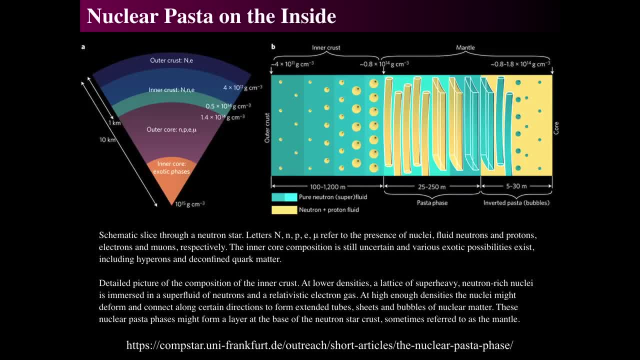 upper, upper level, But between the mantle and the inner crust, You start with these pure neutron fluid, which is the greenish area, And you have a neutron proton superfluid. So you have pure neutrons moving around And then a neutron proton fluid. 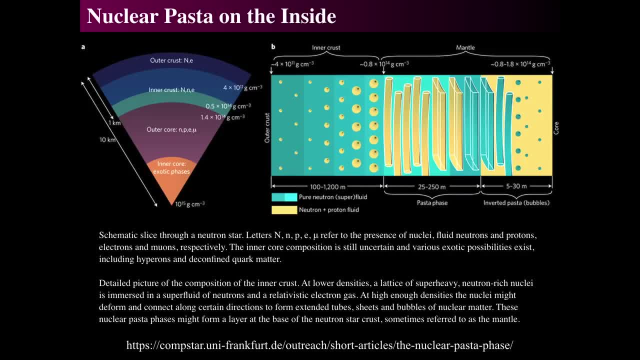 that's in the yellow dots, And eventually those things become larger and larger, Because the proton neutron fluid has to actually get pushed together at higher and higher densities. Eventually the neutrons and protons become stretched into a pasta-like phase, Such that you have just 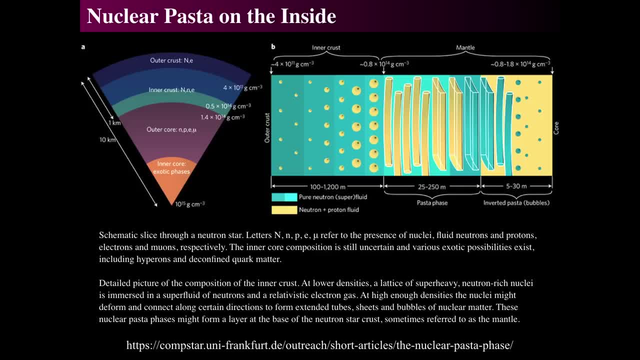 neutrons and protons in like tubes And that's their phase. So it's like a, like an atomic nucleus in the form of a cannoli Or a pasta, Or a mastocci Or a or a ziti. 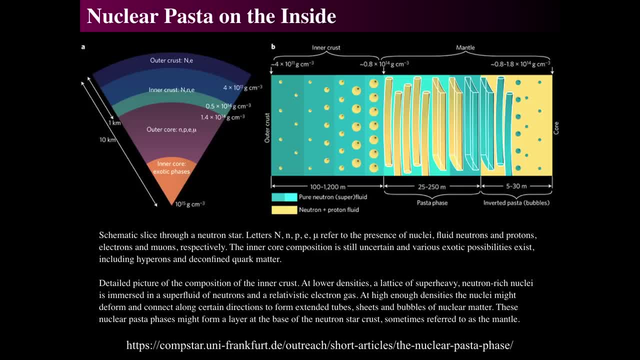 And deeper in the nuclei then form sheets Like lasagna sheets of nuclei. So you have an atomic nucleus in the form of a of a lasagna pasta And deeper in you start to swap it out And it becomes pure neutrons. 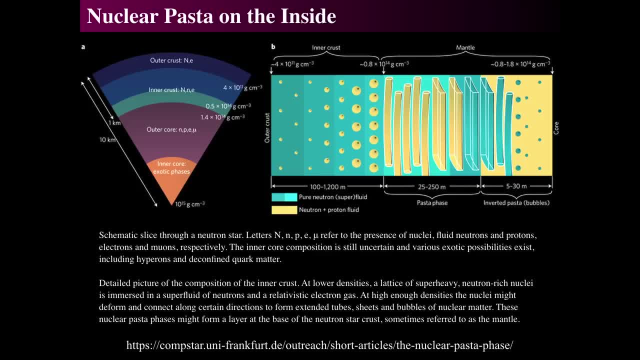 in the core Or and with some isolated protons. But then eventually you don't get any more isolated protons Because the density is too high for individual protons and electrons to exist And they're forced into neutrons. So it flips. 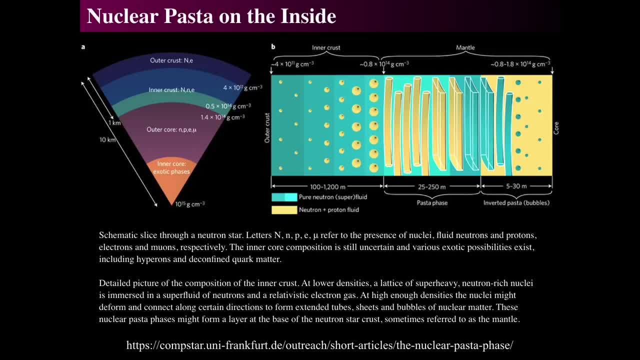 And you have pasta, a lasagna pasta, of just pure neutrons, And then it becomes a pasta of cannoli, of pure, of inverted pasta, Where then you eventually get down to a pure fluid of neutrons and protons in the core. 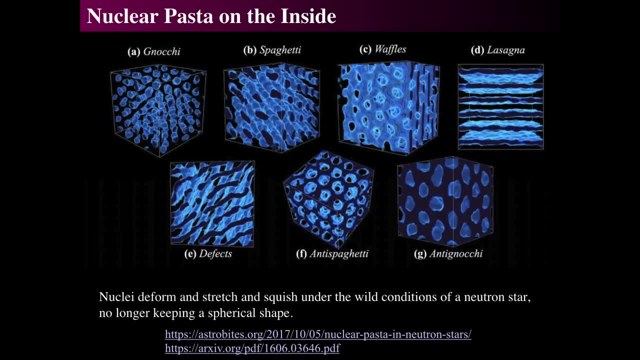 So you have these really strange states, Very, very, very strange states, And they go into exactly how they look and how they shape And it's a fascinating article. I invite you to go to it. Hit that Astro Bytes article that I put on the link there. 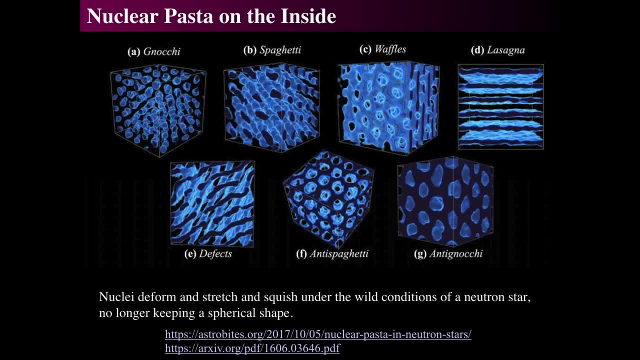 It shows you what the various things look like, But basically the nuclei deform, They're no longer nuclei. The strong nuclear force has very strange behavior in these densities And the individual protons and neutrons bind together not as spherical nuclei but as spaghetti or waffle. 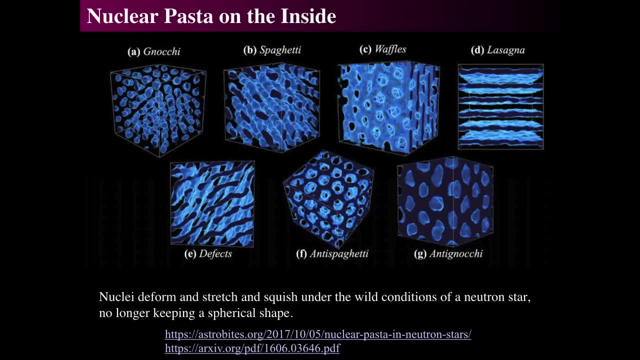 or lasagna type nuclei. So we no longer have anything that looks like oh, this nuclei with next to that nucleus. No, The nuclei are basically huge numbers of protons and neutrons that form spaghetti and waffle type structures or lasagna type structures. 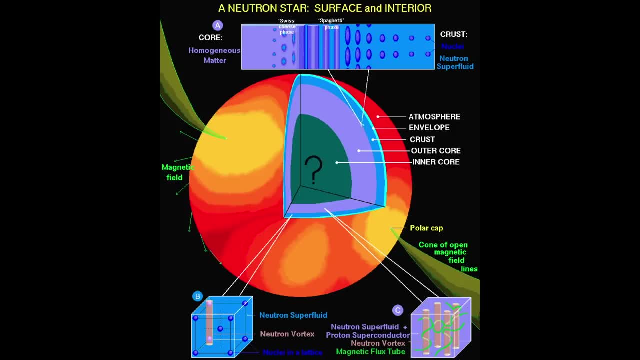 which is really strange. And so then we get this strange, strange, strange of appearance of a neutron star itself And where you have this tiny atmosphere, a crust and an inner crust and who knows what's going down in the core, as the neutrons and everything. 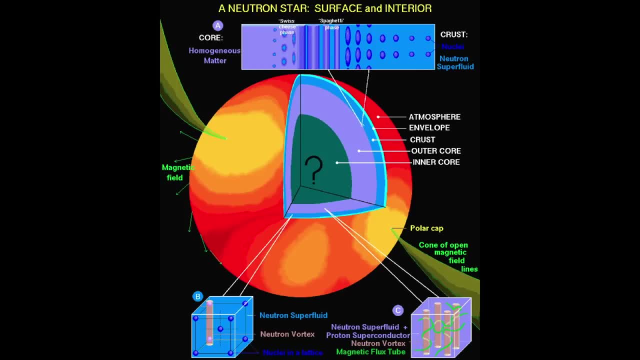 break down to become quarks and individual quark things And neutron stars are really hairy- is the end thing. Nobody really knows what's going on inside of them. They're incredibly hairy objects, but they're the most exotic possible state of matter in the cosmos.